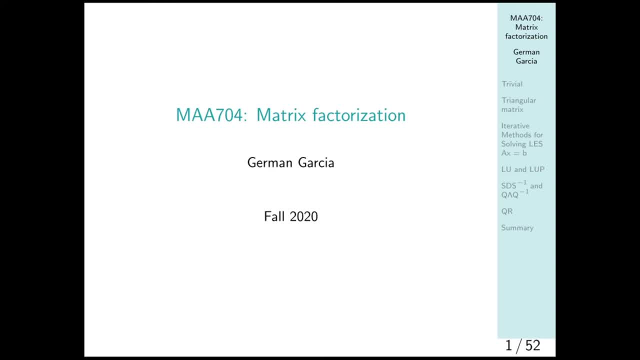 All right, hello everybody. Welcome to Applied Matrix Analysis course code MAI704.. My name is Germán García and in this first lecture we are discussing matrix factorization. In today's lecture we are going to be seeing different types of matrix factorization, from QR to Cholesky and many more. We're going to be discussing interesting. 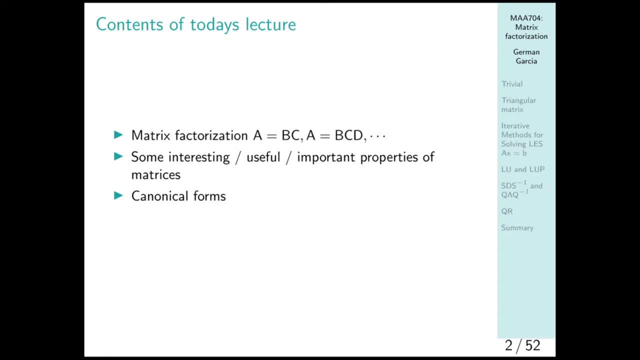 useful and important properties of matrices, Among others, we will discuss what actually allows a matrix to be factorized or decomposed, and also we will discuss some canonical forms like Jordan or QR form. Now, why matrix factorization? You may be asking, Rewriting a matrix as a product? 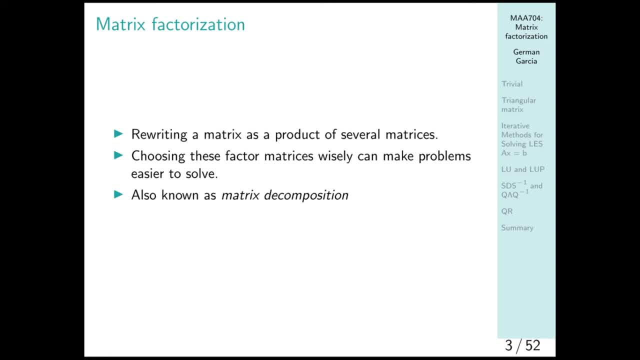 of several matrices have a certain set of advantages. This is especially notorious if the matrix is in the matrix. When you are working with matrices, you can see that the matrix is very large and can be divided into several different matrices. You can see that the matrices are huge, like in three. 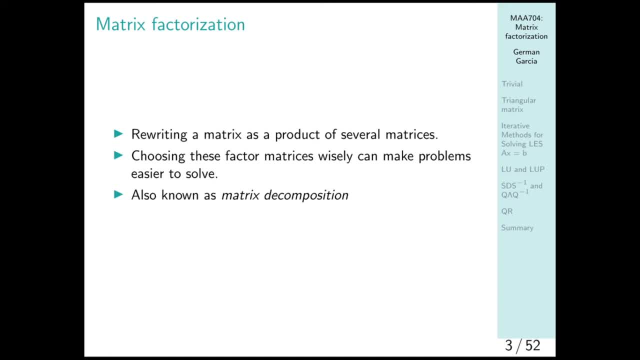 dimensions or four dimensions. This may not be such a big of a difference in terms of work, but when you're working with a 10 000 x 10 000 matrix of data, rewriting it as a product of different matrices can actually save you a lot of computational time. so making problems relative to 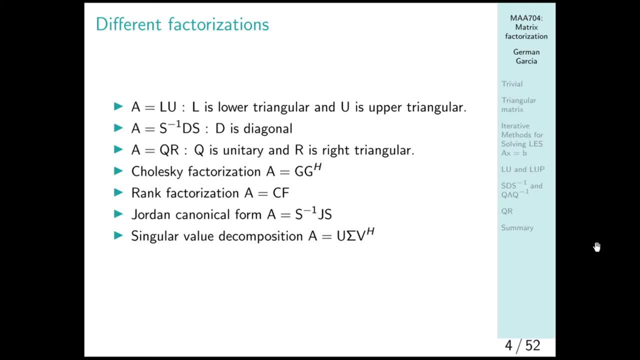 set data much easier to resolve. This is also known as matrix decomposition. have different types of decompositions: LU decomposition, lower triangular times, upper triangular. Another type we have is diagonalization, where there is a change of basis that allows us to rewrite the matrix as a diagonal matrix. QR factorization, which is the product of a 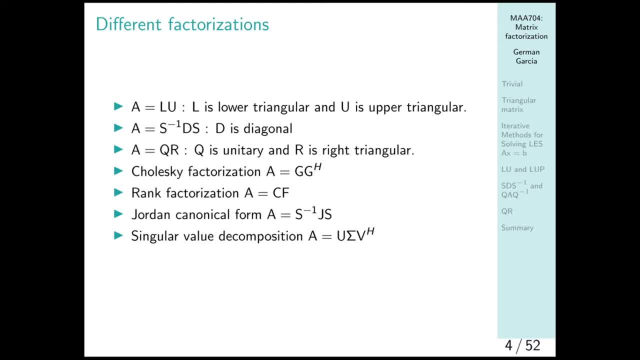 unitary matrix times a right triangular matrix. Cholesky factorization, where we are using Hermitian properties for the matrix. Raft factorization, Jordan canonical form, which is a generalization behind the concept of diagonalization, And we will also be seeing singular value decomposition, why it's used Now. 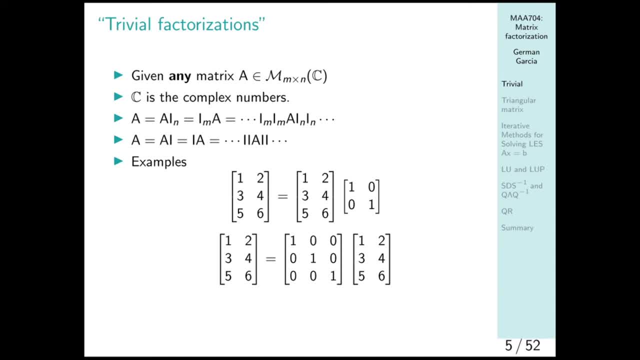 we're going to begin with some trivial factorization. For now we're going to suppose that E is an m times n matrix with complex entries. Of course you have an m times n matrix with complex entries. You have an m times n matrix with complex entries. 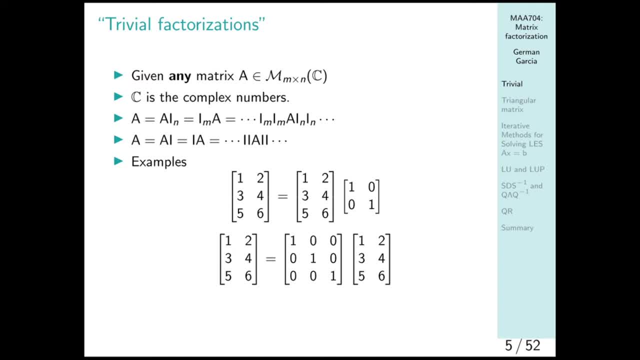 You have an m times n matrix with complex entries. Of course you have an m times n matrix with complex entries. Of course you have an infinite amount of factorizations. if you multiply at right and at left by the proper identity matrix, You have an infinite amount of times you can multiply by an identity matrix. 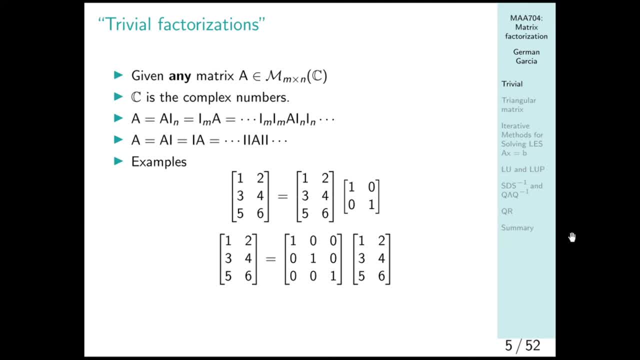 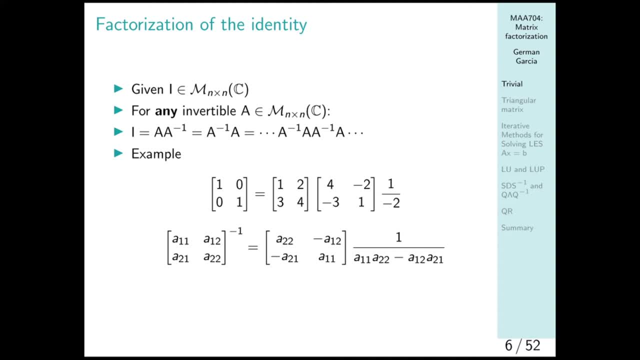 but this is absolutely uninteresting, right? However, factorizing the identity itself is actually quite interesting, a quite interesting problem. We know that for any invertible matrix, the square matrix, namely a square matrix whose determinant is different than one, the identity can be written as a sequence of a matrix times its inverse. 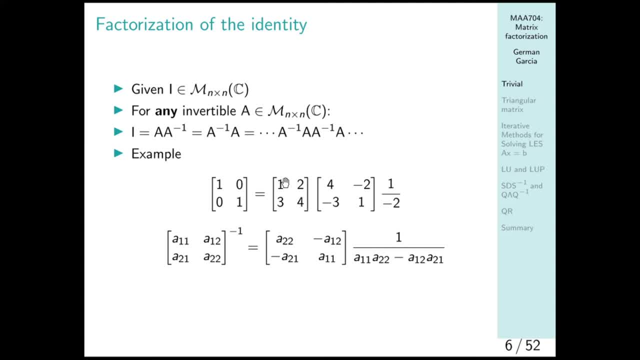 For example, we have this with this matrix: one, two, three, four, an old-time classic- and this will be its inverse. don't forget to multiply by minus one half, and this is the general formula for invertible 2 times 2 matrices. 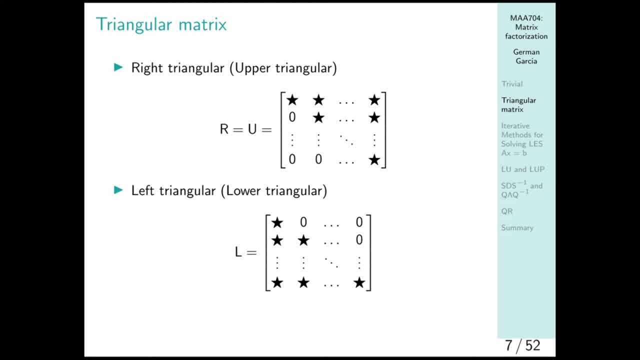 Now we have to talked about triangular matrices. What is a triangular matrix? Okay, we'll say a matrix is triangular if they have non-zero values in the diagonal and then over the diagonal there are zeros and under the diagonal there are no zeros. we are 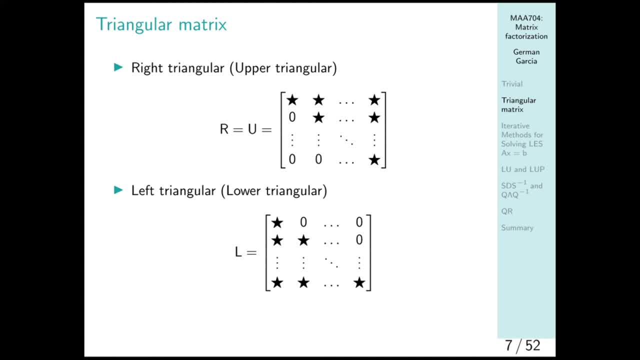 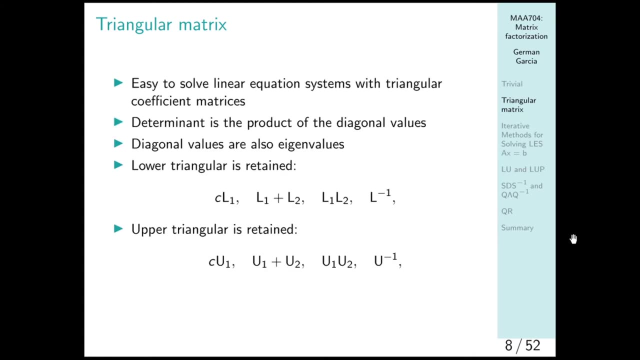 talking about lower triangular. and if it's the opposite- zeros under the diagonal and non-zeros over the diagonal- we'll talk about upper triangular matrices. One of the main advantages of this is that solving systems that involve triangular matrices is trivial, right? I mean you substitute the. 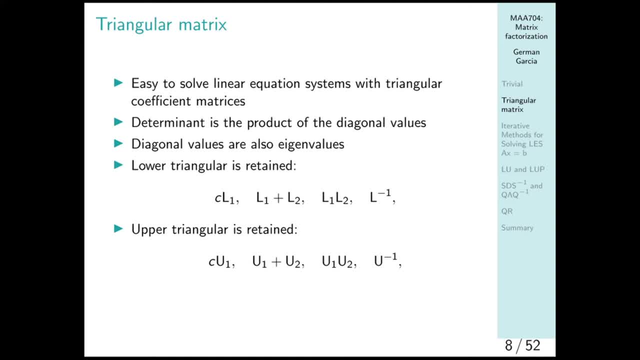 first unknown, and then it goes down and down and down or up and up and up, depending on the matrix you choose. So another advantage of triangular matrices is that it's a determinant. it's actually the product of the diagonal values and you 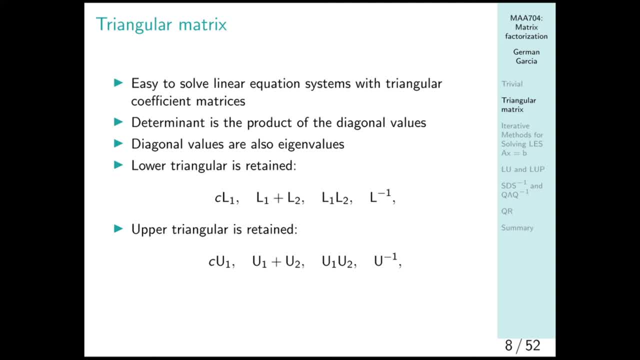 need no complicated formulas, you just multiply everything in the diagonal and this is it. Additionally set elements are the eigenvalues of the matrix. so again, we don't have to calculate characteristic polynomial and solve the characteristic equation with the corresponding possibility of making a mistake. Again, lower triangularity and 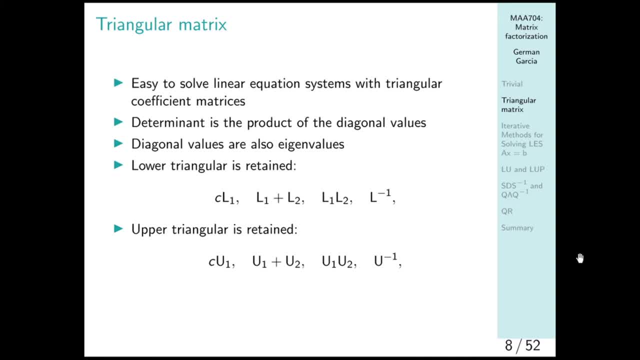 upper triangularity are linear in the sense that they respect product by complex numbers, they respect sum, so they respect linear combination. but also the product of triangular matrices is triangular and the inverse of a triangular matrix is triangular. This is especially important. Now, a different type of triangular matrices are: 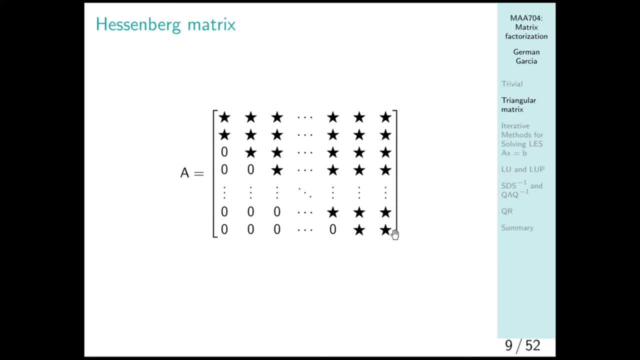 Heisenberg matrices which, as you can see, has non-zeros in the diagonal and have non-zeros right under the diagonal, but all the rest are zeros. This is almost triangular. One of its interesting properties is that if you multiply it with an upper triangular matrix or a lower Heisenberg matrix, you 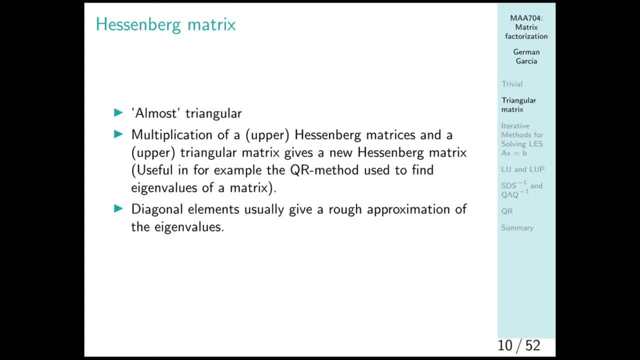 multiply it with a lower triangular matrix, it gives you a new Heisenberg matrix. This is especially important when you're working, for example, with the QR composition of matrices, where Heisenberg matrices come in handy Also. this could be useful sometimes. The eigenelements usually give a rough approximation of the. 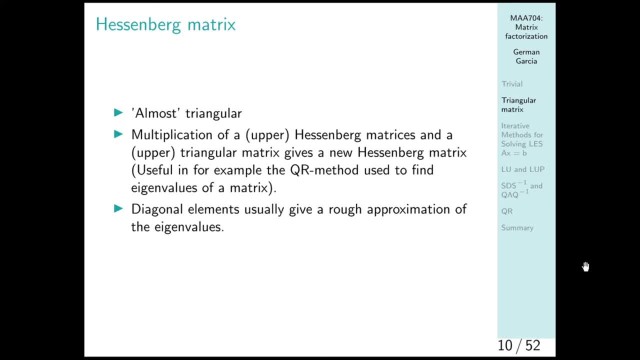 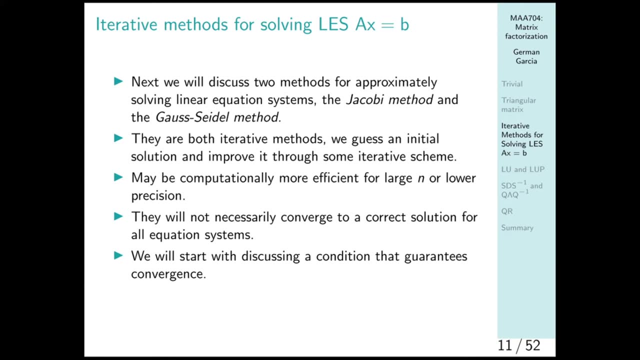 eigenvalues. At some point it will be hard to do a lower-upper factorization that gives us the exact eigenvalues, but we can get a rough enough approximation, which sometimes is actually more than enough. So the main approximation to factorization, as we have said, 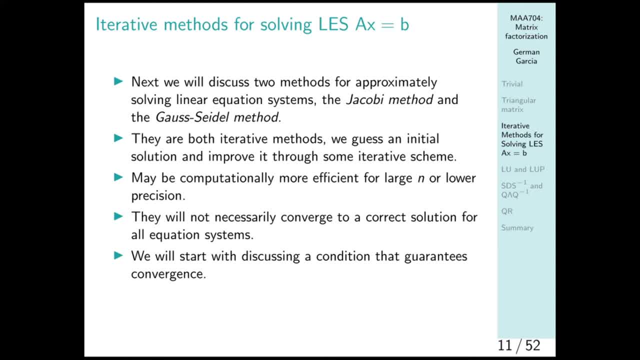 before is to solve complicated linear problems or to solve linear products in very high dimensions. In order to do that, we're going to first approach the Jacobi method and the Gauss-Seidel method, which are the the two introductory methods to matrix factorizations. They're both. 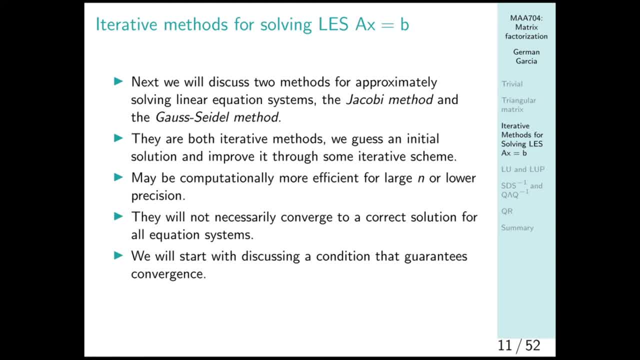 iterative. so it means we guess an initial solution and then we use an iterative scheme to perfect it, to polish it until we get to the actual solution. The reason why we do this is that it will be computationally more efficient for large numbers, for a large dimension of the matrix, or if we don't. 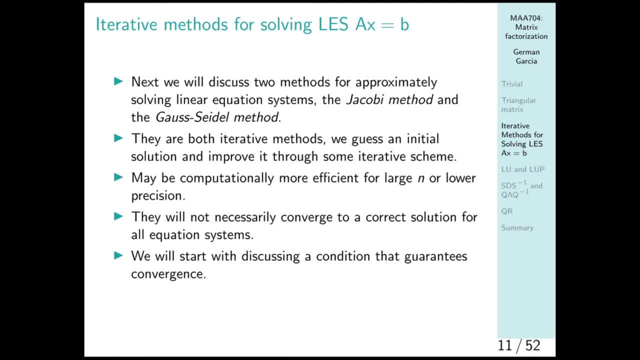 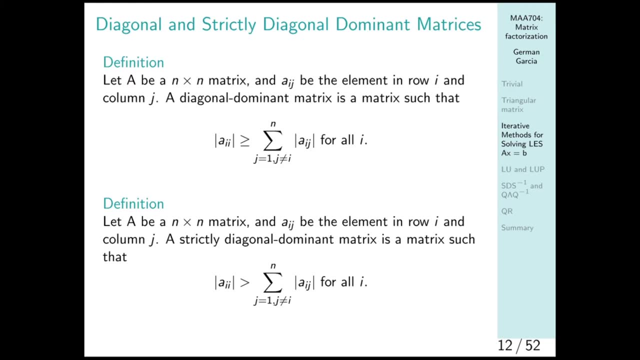 require as much precision. we can just stop the iterative process at any time. Unfortunately, it doesn't have to converge to a correct solution. so first of all, we're going to see some conditions that actually grant that. So we're going to let A be a square matrix and we will call it. 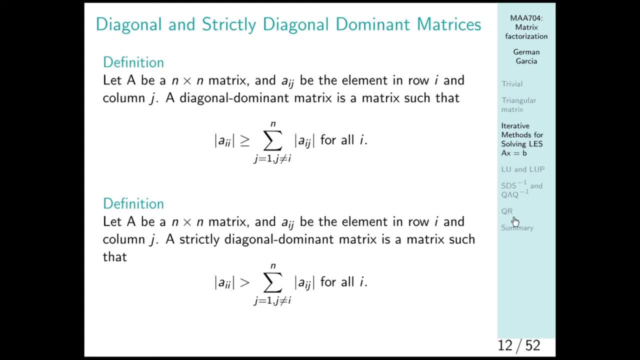 diagonal dominant if the absolute value of the elements in the diagonal is greater or equal than the sum of absolute values of the rest of the elements in that row. So the diagonal is bigger in absolute value than the sum of the absolute values in the rest of the row. 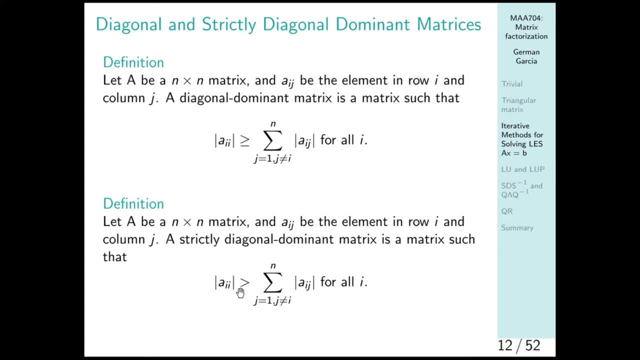 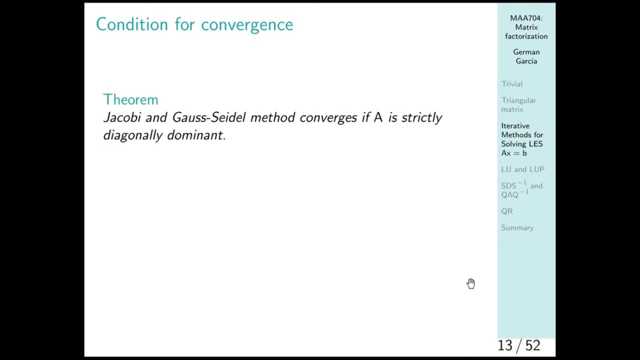 If, instead of being greater than equal, we require inequality to be strict. you're talking about strictly diagonal dominant matrices. So first theorem: both Jacobi and Gauss-Seidel method converge if A is strictly diagonally dominant. Now, this implication is only one direction. it doesn't help the other, so it. 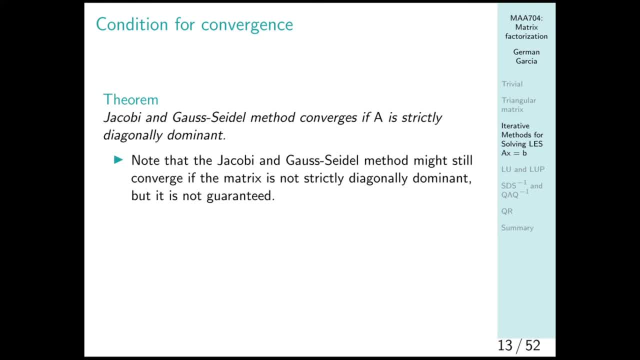 means if the matrix is not strictly diagonally dominant, the methods might converge, but it's not guaranteed that they will, For instance, if for matrices that are diagonally dominant, there are some really interesting examples in which both methods converge, but they do it so slowly that it's really 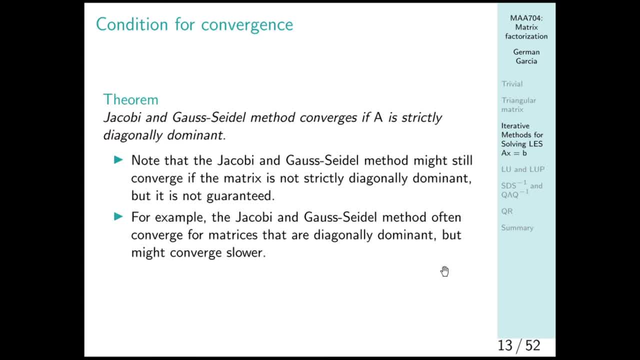 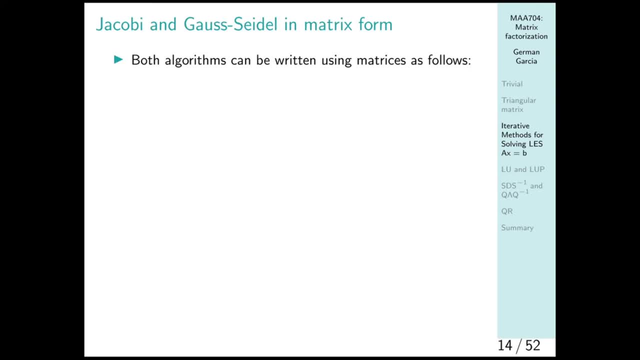 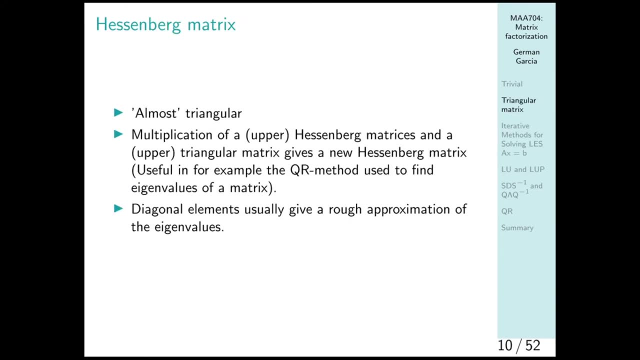 not relevant. So the first thing we will search for is strict diagonally convergence dominance. sorry, Now both algorithms can be seen in this form. Remember that what we are trying to solve is the linear equation system: A: x equal b. matrix times column. vector equal column. 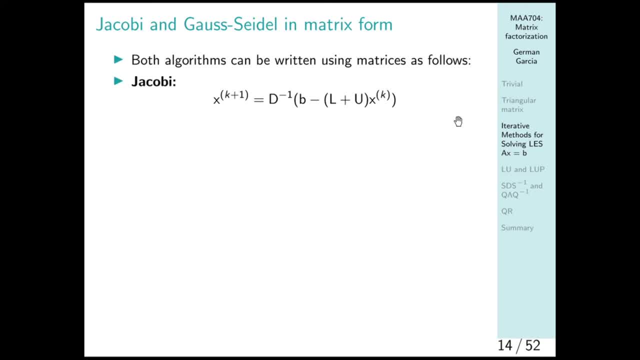 vector, And so the Jacobi method states that the x vector in the k plus 1th step will be equal to this Little monster. And regarding the Gauss-Seidel method, we use this formula. Here what we have done is the trivial triangular decomposition, namely A equal L plus D plus U, when we separate. 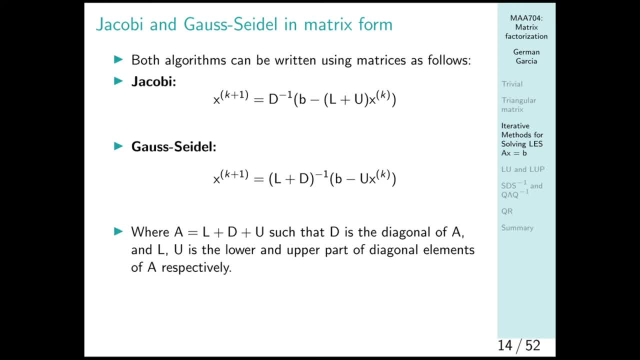 the diagonal, the elements below the diagonal and the elements above the diagonal. That's something that we can always do with a square matrix. Of course, this is not a product. this is a sum, But still it will do. Now, this is very important. These L and U that we are using here are not the same L. 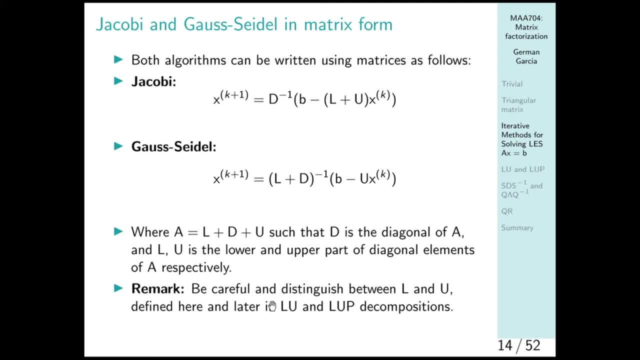 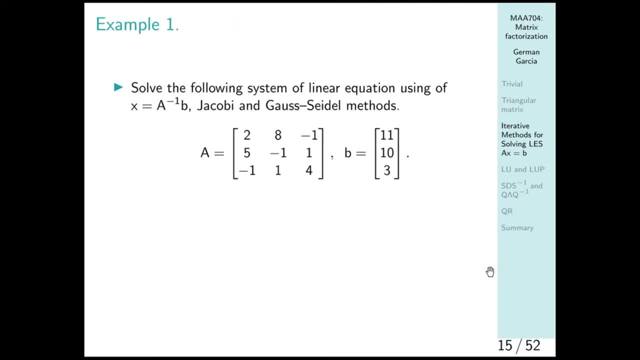 and U that we will use in LU and LUP decompositions. Namely, these are summed and these will be multiplied later. So we're going to see a small example. We have this equation system: three equations, three unknowns. We can use this Matlab code to help us get to the answer: Proposeless. 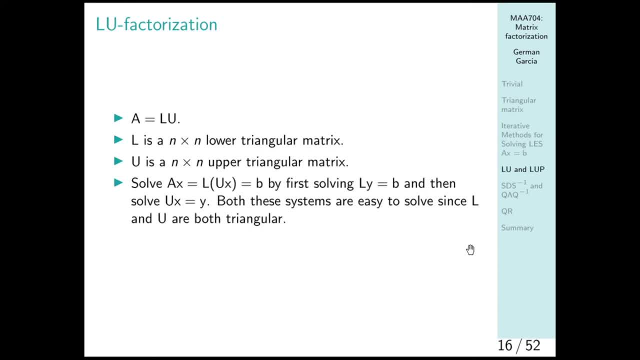 exercise Now regarding L-U factorization. what we want is to divide the matrix in the product of two square matrices in which L is lower triangular and N is upper triangular. So in this sense, the system AX equal B can be seen as L times UX equal B. 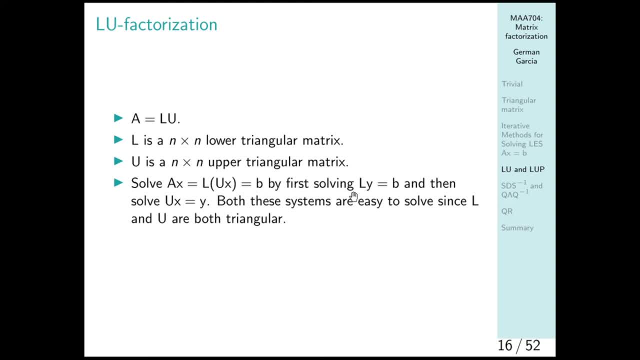 So what we can solve is a second system, namely L times a. vector Y equals B and we have this vector Y, we move it here and we solve UX equal Y. These systems will be immediate because both L and U are triangular matrices. 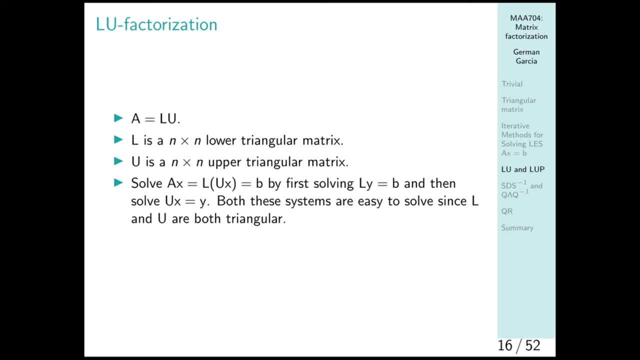 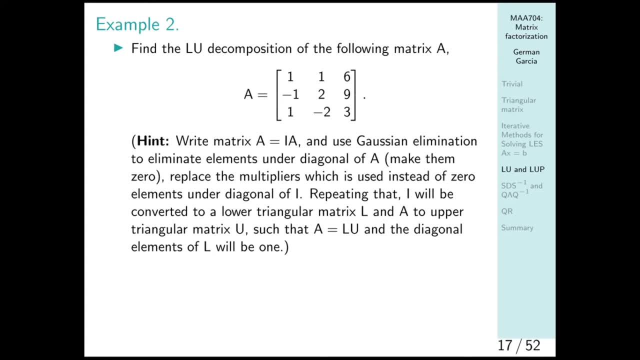 Of course, this will not be as helpful with a three times three matrix, but when you get 10,000 unknowns, things change a bit. So we're going to, We're going to try and find the L-U decomposition of this. 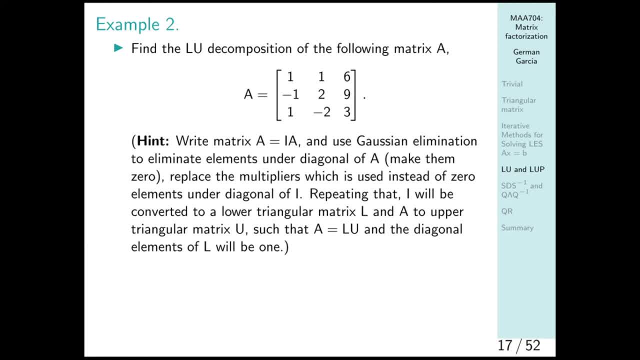 And this is mostly the method. This is mostly what we do. We're going to write the matrix as the matrix as a dotted bar, and then identity matrix or the other way around, and then do Gaussian decomposition until we get lower triangular in one side and upper triangular in the other. 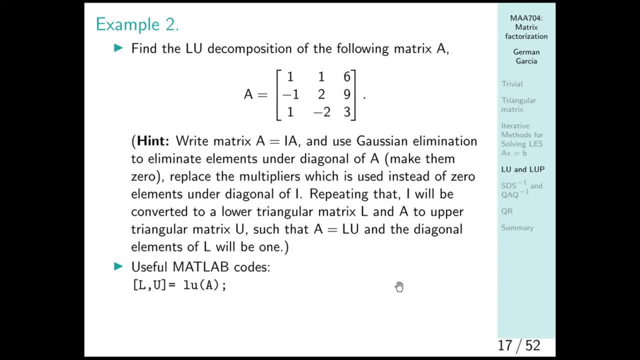 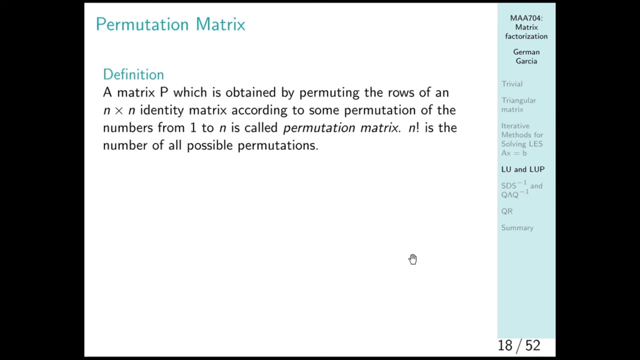 Of course, L-U factorization is almost a standard in MATLAB, so you can actually use comma L-U for that. Now, the problem with this factorization is that not every square matrix has one. This is why we need P. Remember that I've said L-U-P decomposition a few minutes before. 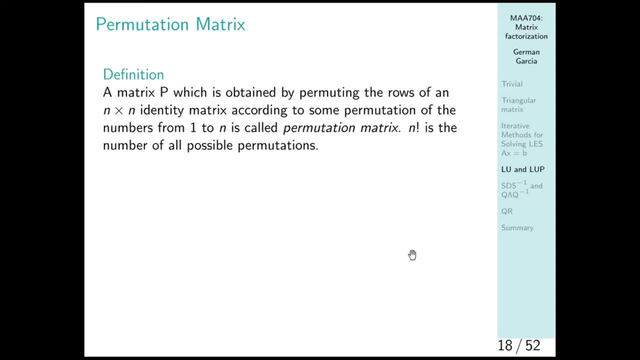 The reason is We are using a permutation matrix. A permutation matrix, one of N-factorial- is a matrix that has the columns of the identity matrix but swapped. So these matrices work in this way. If you multiply at the left they swap rows. 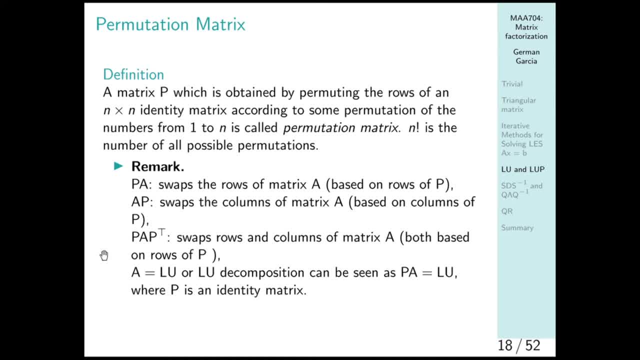 If you multiply at right, they swap columns. If you multiply by left and then by right, transpose you swap both rows. If you multiply by left and then by right, transpose you swap both rows. If you multiply by left and then by right, transpose you swap both rows. 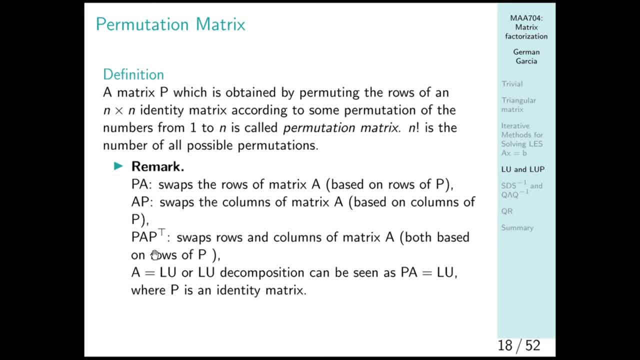 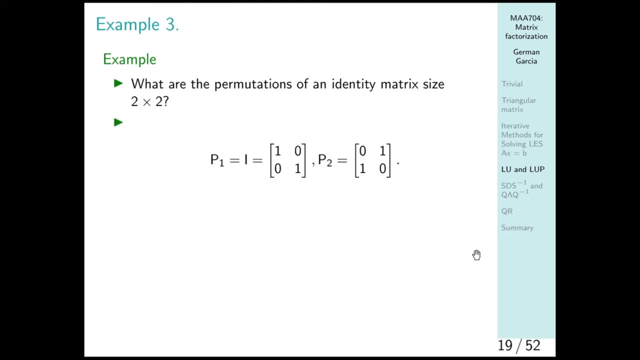 Finally, this factoring can be seen as another square matrix, with its rows or columns permuted equal L-U. Of course, this is Identity Matrix. So what are the permutations of the identity matrix of size 2?? So what are the permutations of the Identity Matrix of size 2?? 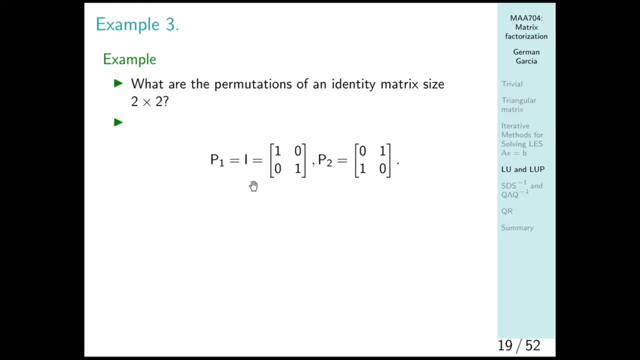 Well, we have 1 and 15 plus 13.. We can at least translate it into four units. we can permute either rows or columns and we get p2. that is mostly this small one over here. How many permutations do we have for the identity matrix in? 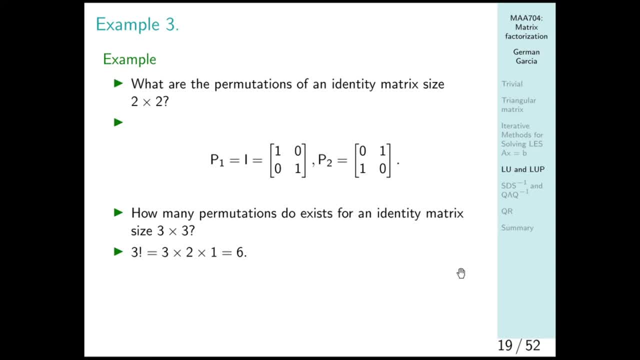 dimension 3? 6.. We have three options for the first column, then two for the second and one for the last. The same thing with rows. And this is a true question. Can we make the matrix A in example 1 strictly dominant? I'm going to go back to example 1.. 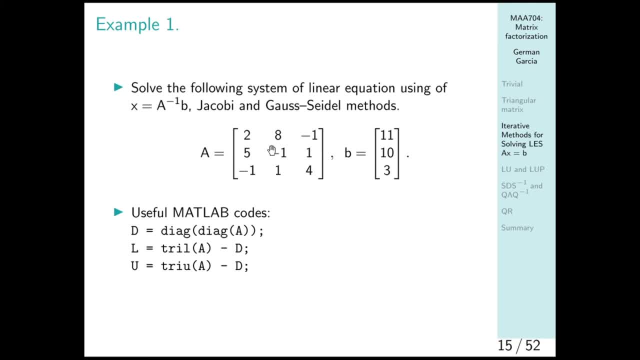 This one. Can we do a permutation of columns that turns this into strictly diagonal dominant? We can see that if we swap columns 1 and 2, then the 8 becomes a part of the diagonal and the 5 becomes a part of the diagonal And then we have a strict diagonal dominance. 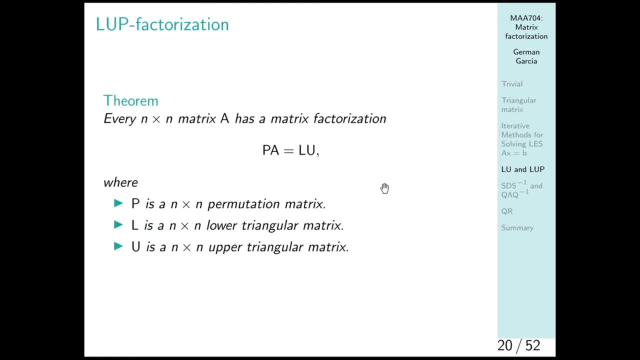 And so we arrive to this, this important theorem about LUP factorization. It says that every n times n matrix A has a matrix factorization where the matrix with a certain row or column change has, can be expressed as the product of a lower triangular matrix times an upper triangular matrix. 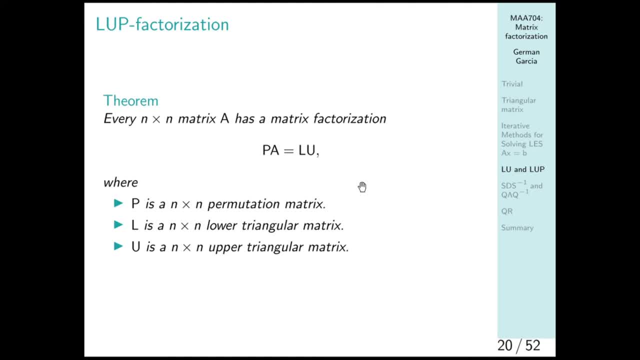 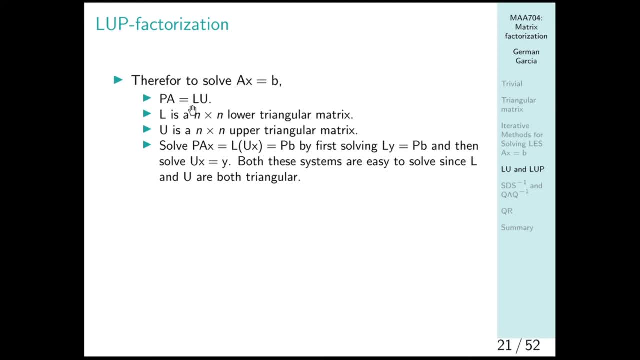 This one is incredibly important, Because what can we do with it? We can, if we want to go to this system, we can apply this equality, And so we multiply both sides by b, Which we can do, since this is a square matrix, this is a vector with the same size, And we have is PAx equal pb, but PA is LU. 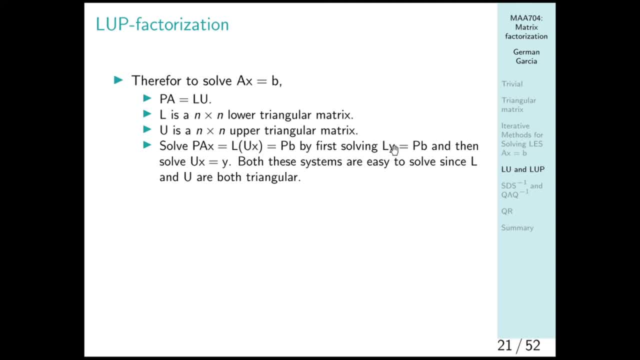 So we can do the same trick as before. We change ux by a vector y, we solve ly equals pb, where this is known, and this is lower triangular. And then, when we have values for y, we solve ux equals y And the system is upper triangular, so it solves immediately. 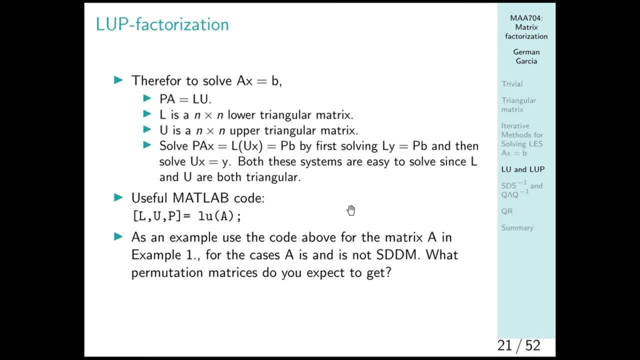 So one thing you can do at home is use this code for matrix A, for the matrix in example 1. And check for which cases A is and is not strictly diagonally dominant And, of course, tell me which denotation matrices do you expect to get. 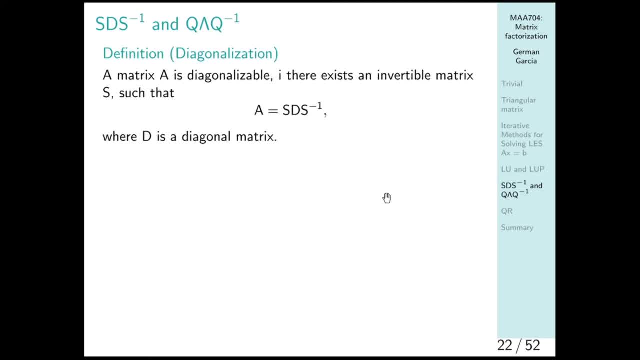 There are at least two that should do the trick. Now, I guess all of you have at least some background in linear algebra. In that sense we will say that A matrix A is diagonalizable if there exists an invertible matrix A, such that the matrix is basically a matrix, a diagonal matrix, and the inverse of this matrix. here 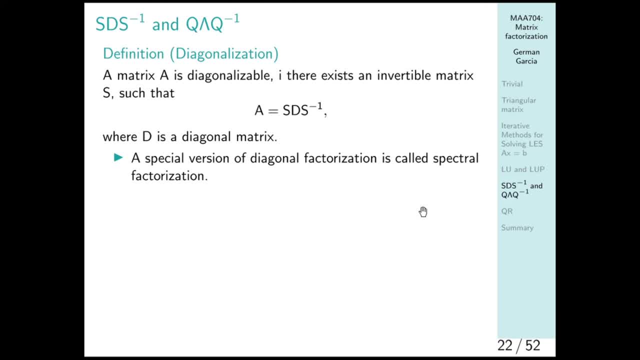 This is called a change of basis in linear algebra, when we simply look at the matrix from a different perspective And it happens to become diagonal. So There is a special version of this factorization which is called the spectral factorization, And this is the one we know from the first course of linear algebra. 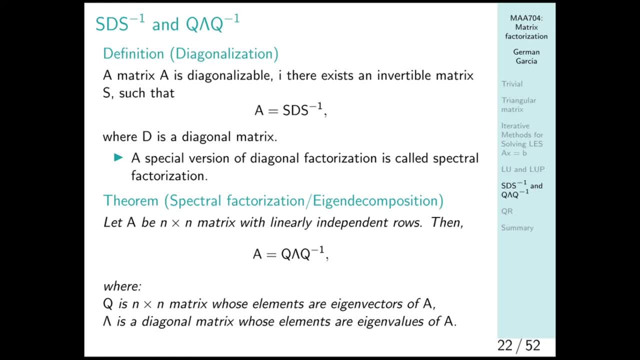 An n times n matrix which has linearly independent rows, slash, columns. slash is invertible. It can be expressed as the matrix of eigenvectors times the matrix of eigenvalues, which is diagonal times the inverse of the matrix. This is a perfectly common example of factorization. 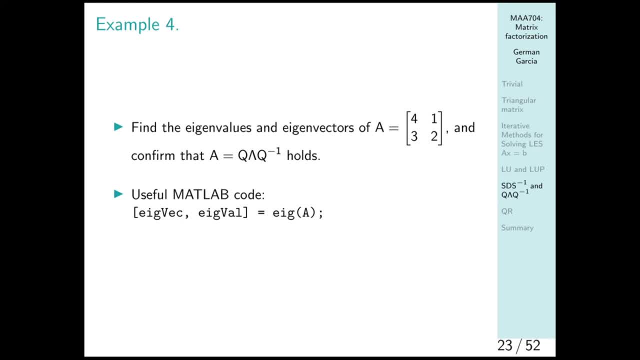 So eigenvectors and eigenvalues. you can calculate them using MATLAB, here using this command. And please, when you're at home, take some time, Put this in the comments, Put this into MATLAB and check it. Now a slightly more general form of the eigenmatrices, as sometimes diagonalization is not possible. 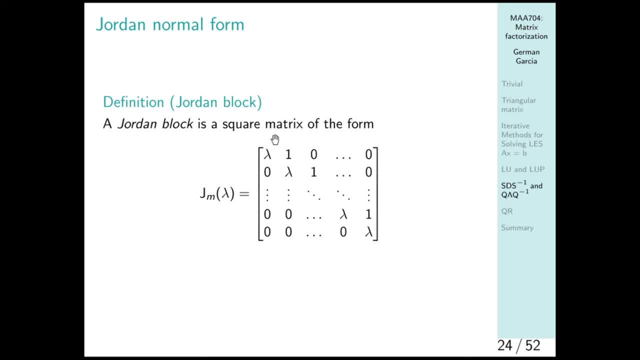 is the division in what is called a Jordan block. A Jordan block is a matrix with m equal to the multiplicity of the corresponding eigenvalue that has that exact amount of iterations of the eigenvalue in the diagonal and the upper diagonal is all 1s. 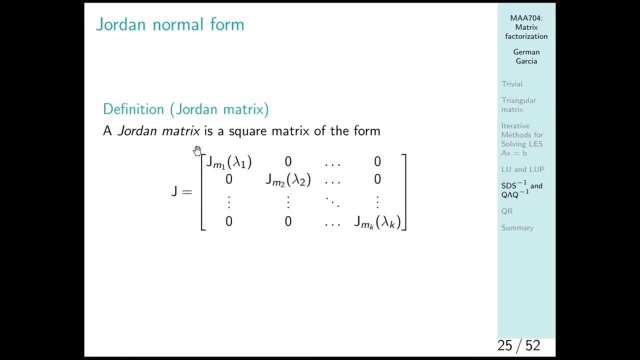 So we can say that a Jordan matrix is a matrix that has Jordan blocks in the diagonal, namely a block with eigenvalue lambda 1,, here a block with eigenvalue lambda 2, and all the way until we get to all the eigenvalues. 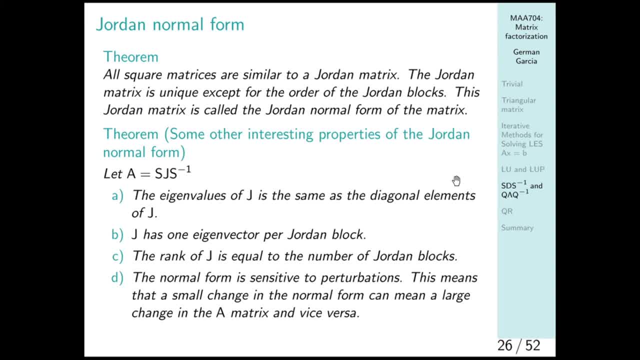 So this is the good one. All square matrices are similar to a Jordan matrix, So now we don't have the matrix to be invertible or any other condition. All square matrices are similar to Jordan matrix. Diagonalizable matrices are actually Jordan matrices, but there all the eigenvalues have. 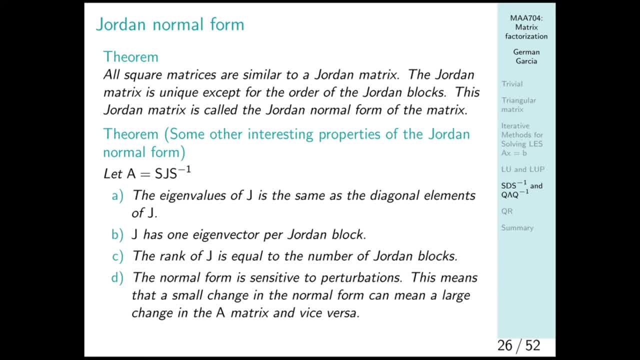 multiplicity 1.. So the Jordan blocks are only one number, namely the eigenvalue. This Jordan matrix is called Jordan, canonical form of the eigenvalue. So this is the Jordan matrix, This is the Jordan matrix. It is an eigenvalue of the matrix in its own right and this is the eigenvalue of the matrix. 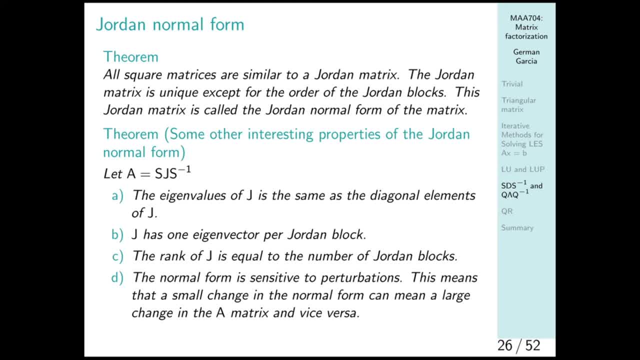 in its own right, The. again, this is actually Jordan canonical form of the matrix, or Jordan norm form. Now I have spoiled to you all these properties, but let's go through them again. The diagonal elements of the Jordan canonical matrix are the eigenvalues. 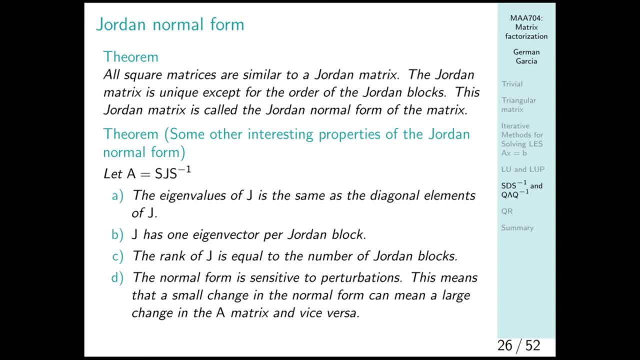 The Jordan canonical framework has one eigenvector corresponding to each Jordan block. The rank of this matrix is equal to the number of Jordan blocks, Unfortunately sensitive to perturbations. this means that if you change, for example, one number in one of the Jordan blocks, the whole value of A can go over the hills and far away. 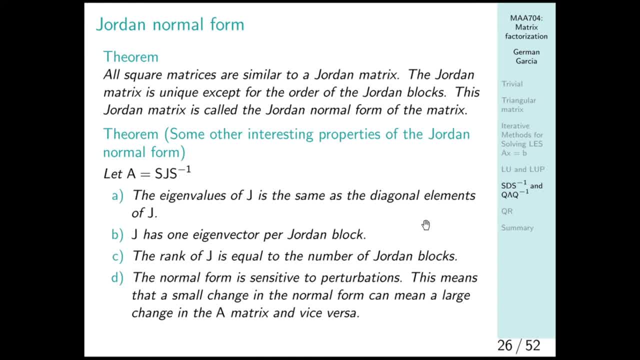 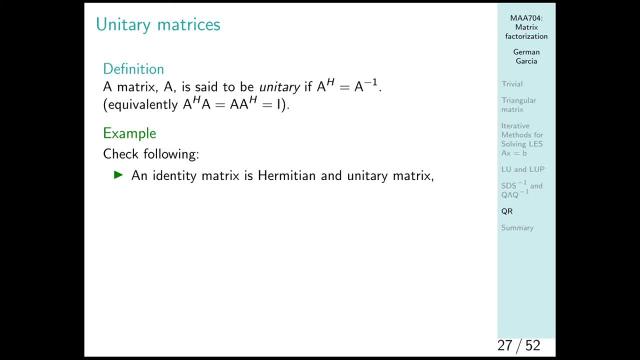 This is what sensitivity means. Now we have talked about the Hermitian conjugate, And so we will say that a matrix is unitary if the Hermitian conjugate is exactly its inverse. So, for example, an identity matrix is Hermitian and unitary. 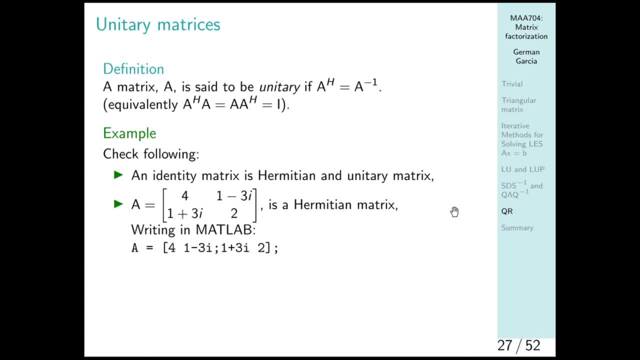 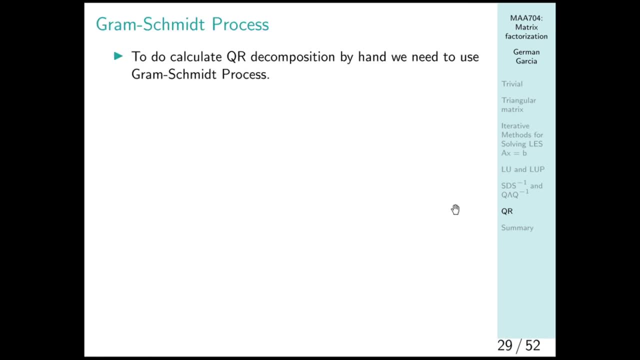 This matrix is Hermitian. Remember that a Hermitian conjugate is the conjugate of the transposed matrix. Of course, this is a unitary matrix as well. So here we have a definition. The Hermitian conjugate is the complex conjugate of the transposed matrix. 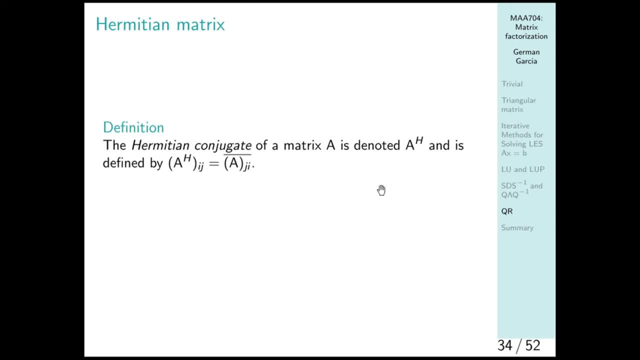 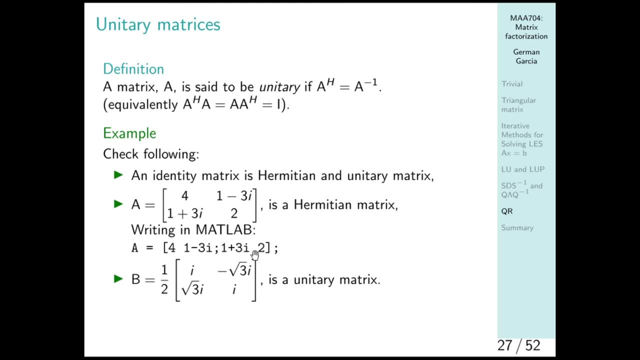 So we swap rows by columns and then y becomes minus y. So these are good examples of Hermitian matrices Here. if you view the transposed matrix, you can see that the Hermitian conjugate is the complex conjugate of the transposed matrix. 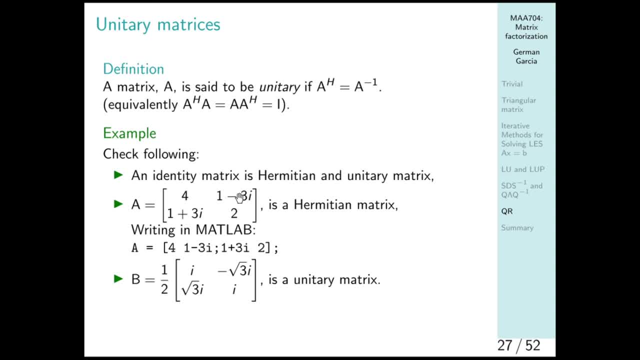 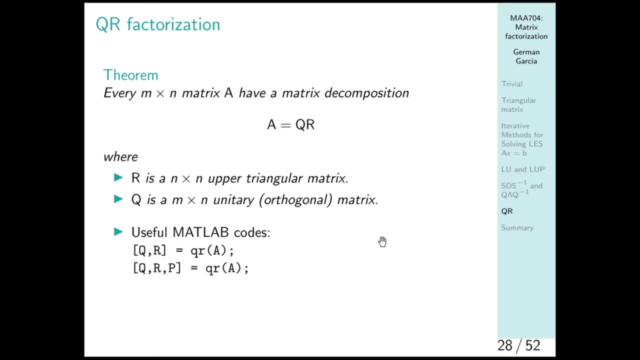 The minus comes here and the plus comes here. But when you take the complex conjugate, this plus becomes a minus, this plus becomes a minus. Now we are moving into a kind of a little bit more powerful method, namely QR factorization. 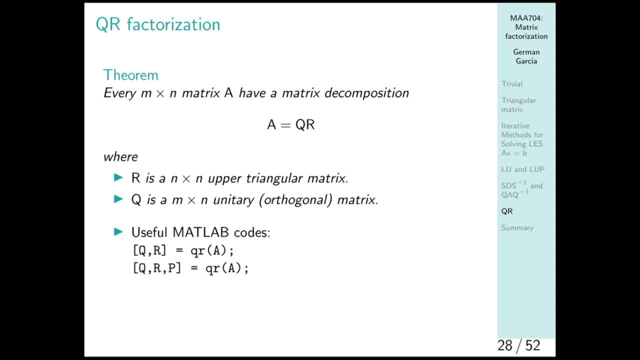 Every matrix, including those that are not squared, admit a matrix decomposition in this form, Where R is upper triangular and Q is a unitary matrix, namely the determinant equals 1.. Of course, at some points, commuting rows or columns can actually be useful in certain terms. 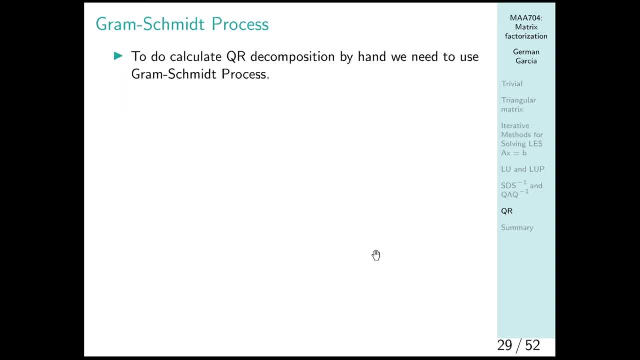 We will see that afterwards. How do we calculate Metrics Q and R? What we are going to do is something you will probably never get tired of, And that's Gram-Schmidt orthonormalization process. So we are going to call every column of matrix A, A1,, A2 to AN. 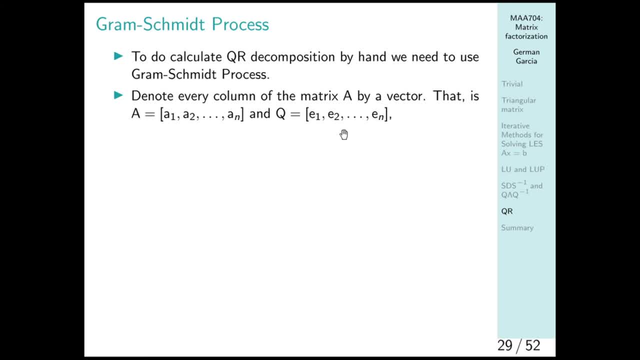 And those of the matrix Q will be named E1, E2 until AN. So we are going to search for a new orthonormal basis With which, whose vectors we will use to build that matrix, matrix Q. So, following orthonormalization process by Gram-Schmidt we have: first vector is A1.. 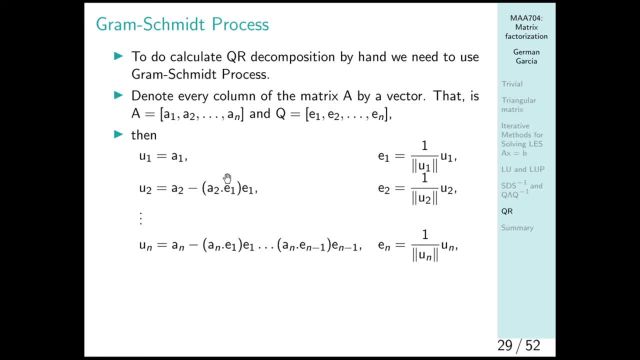 So A1 is A1 divided by its norm, And then we will. we continue iterating this process. Of course this is a 2-norm And here the dot is a normal scalar product. When you take two vectors of the same size against each other, one is transposed. 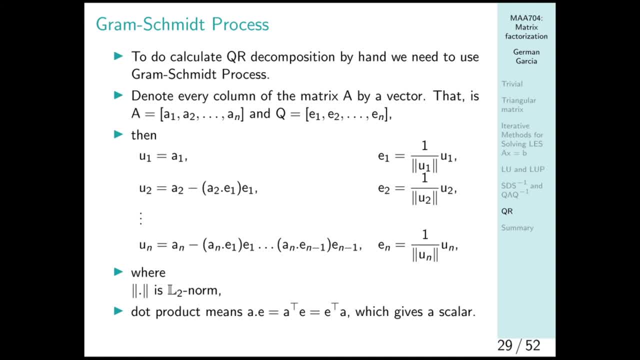 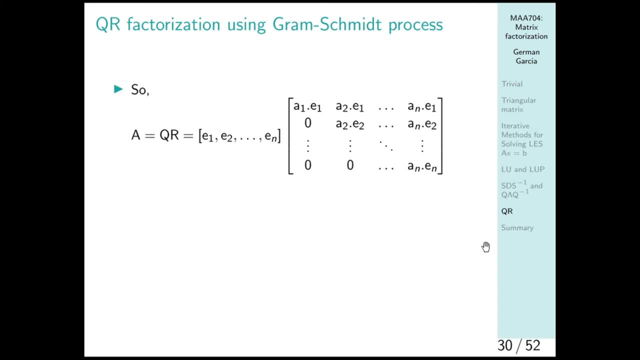 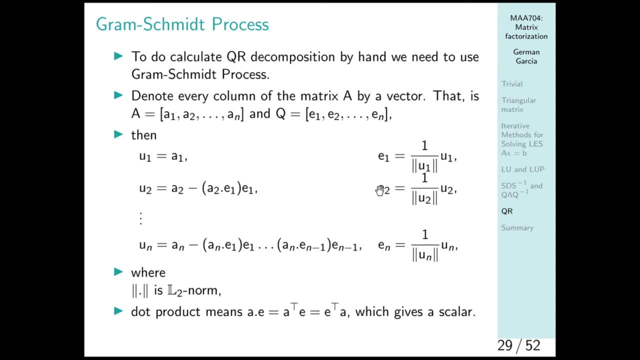 And you multiply first by first and second by second and third by third and so on. So this is basically a number. So what we have in the end is as interesting as these vectors that we have calculated here, Adding matrix Q. 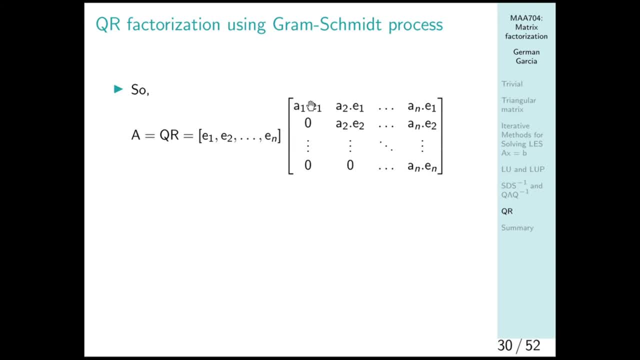 And what we have in the diagonal and over the diagonal is these scalar products over here. So this is way less cryptic than it looked in the first place. right, This one, we are going to do it. So we take this nice matrix which has three vectors. 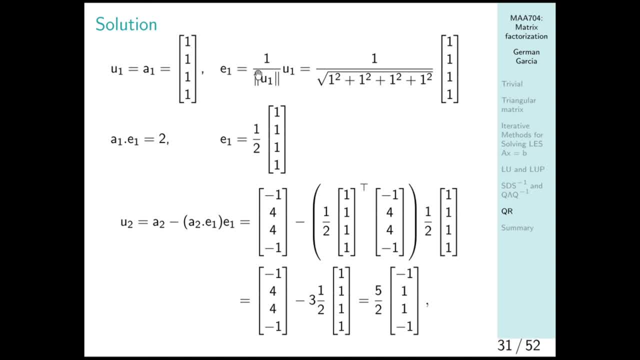 First vector is 1,, 1,, 1,, 1.. So our first column in Q is this, divided by its norm, which is the square root of 4, namely 2.. And so with this we have the first value of the diagonal of R. 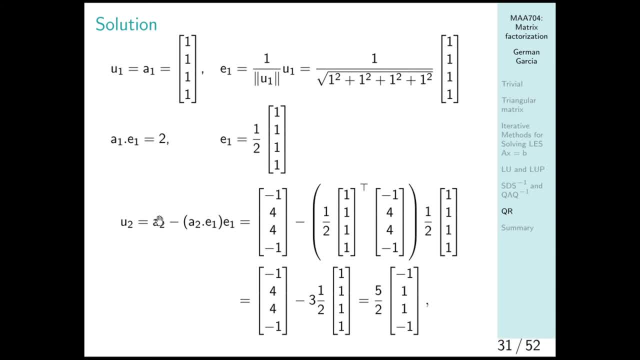 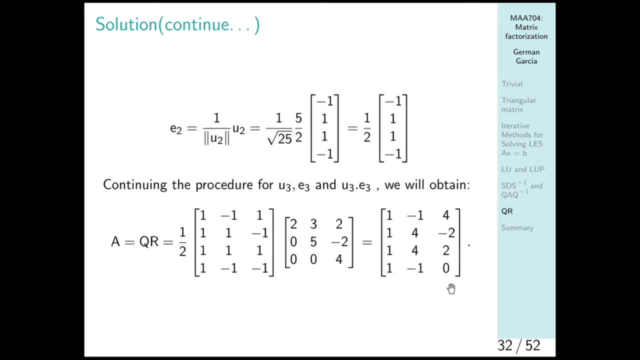 Now for U2, we take the second vector, the second column of A minus scalar product of it, with E1 times E1.. We solve it, We have this one, We'll get this super nice vector over here And we finish for U3,, E3, and the product of those. 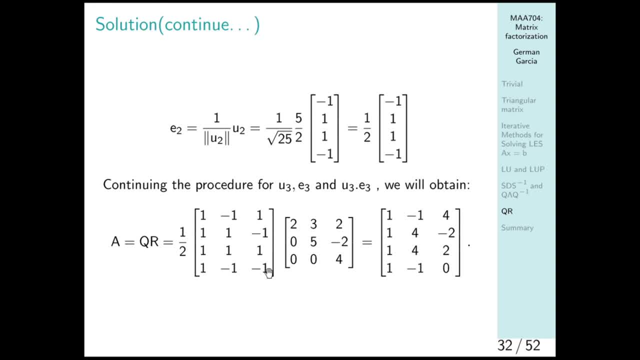 And we get this super nice matrix. Honestly, this is super nice, I mean all at once. What else can you ask for? And, using this scalar product, we have this upper triangular matrix. How do we know that this is correct? 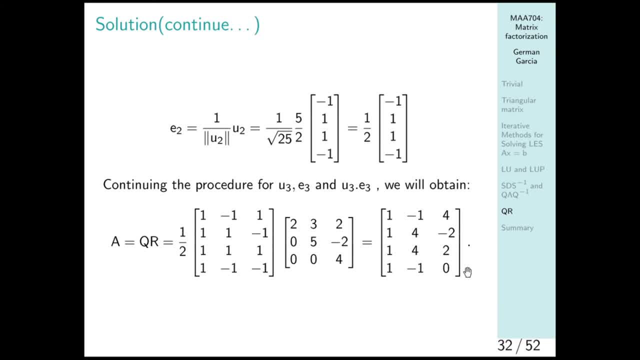 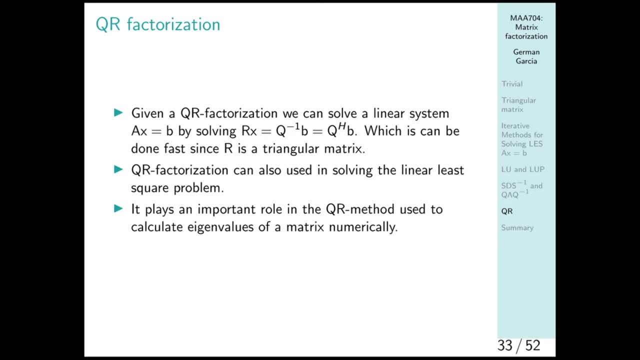 We multiply both and we get back the original matrix. You can use MATLAB to test this one. So what is this useful for? Okay, What we have here is that the system AX equals B can be reduced actually to RX equals Q minus 1 B. 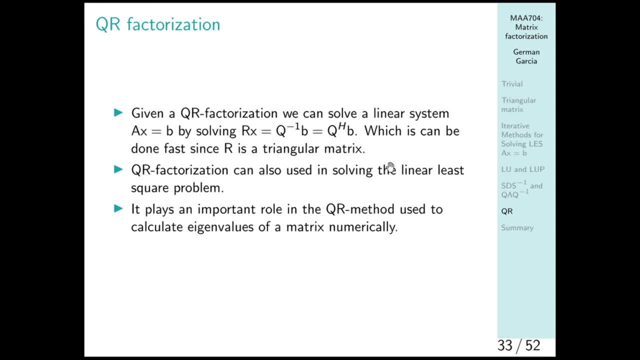 which is Q conjugate transpose B. This we can calculate at any moment. Matrix nice vector, This is known And this is upper triangular matrix, which means this system is incredibly fast to solve Other applications QR factorization has, for example, we can use it to solve linear least square method. 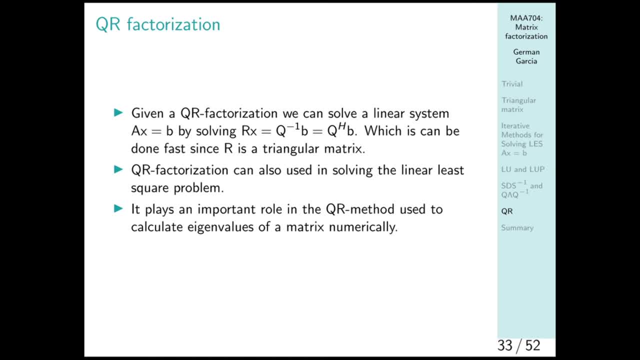 that we will see in a lot of depth later on, And so one of the interesting applications of the QR method is We can use it to calculate approximations to the eigenvalues. Now, I definitely should have put this definition before. 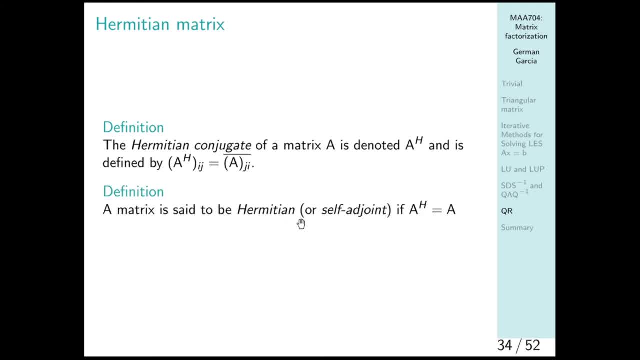 But yeah, the Hermitian conjugate of matrix A is the conjugate transpose. basically, A matrix is Hermitian if it coincides to its conjugate transpose, or in some literature you will see it named as self-adjoint. 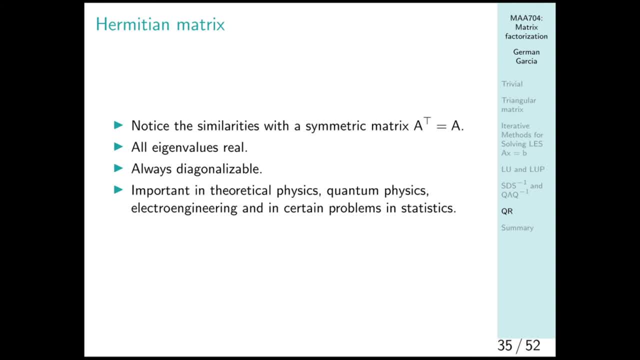 Now, Hermitian matrices are kind of a generalization of symmetric matrices. Namely, all symmetric matrices in real numbers are Hermitian. So interesting properties. all the eigenvalues are real, they're always diagonalizable, and so they are really important in theoretical and quantum physics. 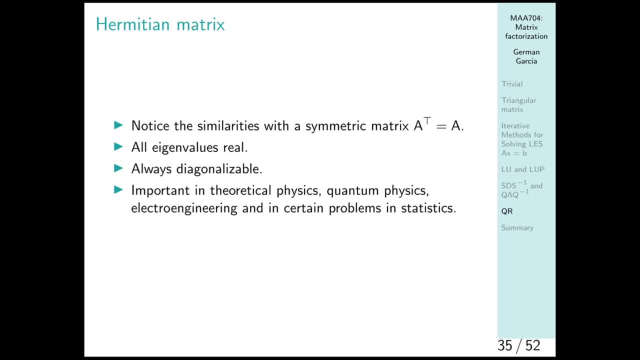 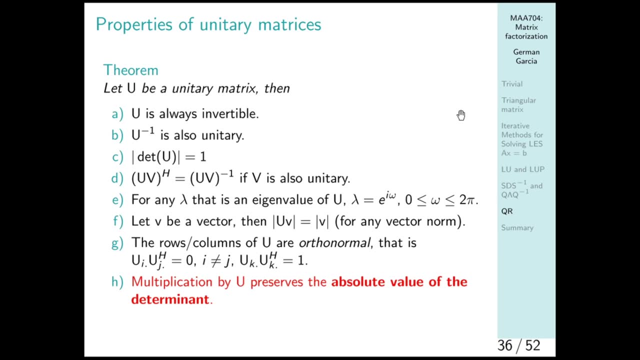 There are problems in statistics that involve Hermitian and symmetric matrices. Biggest example: the covariance matrix of any distribution is symmetric. So that's a certain amount of applications, And so now we're going to talk about unitary matrices. 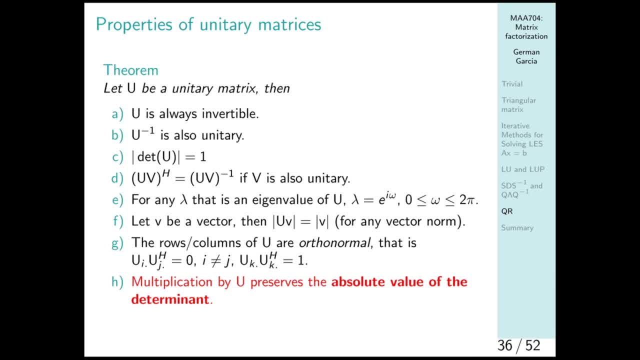 In this case, unitary matrices are always invertible. Its inverse is unitary. They have a determinant 1. If V is also unitary, then the conjugate transpose is its inverse. Wow, this is a good one, This is a really good one. 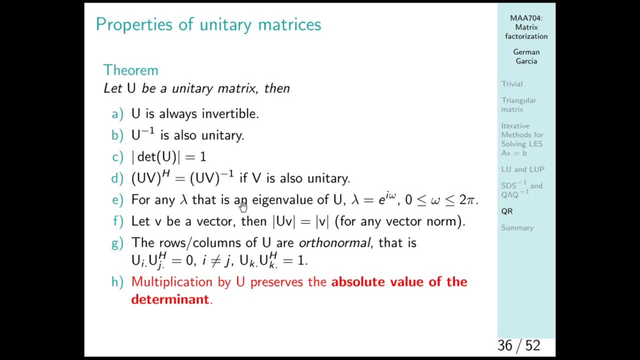 So another good thing is that all the eigenvalues lie in the unit circle, which makes it quite interesting, And this actually means that the norm of the matrix times any vector is preserved. So this matrix is unitary. This is a movement actually. 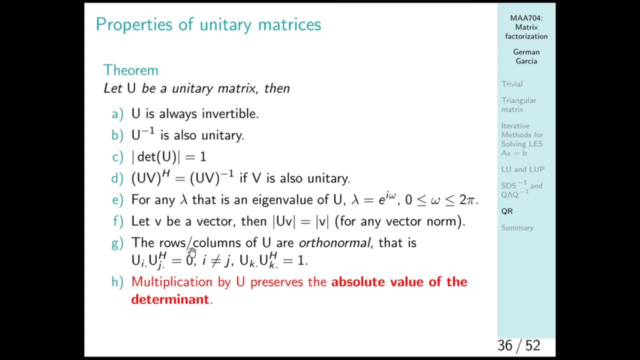 It preserves the norm. And lastly, the rows columns and U are orthonormal. Namely this: once again, the scalar product of different columns is zero, but the scalar product of every column with itself is one. 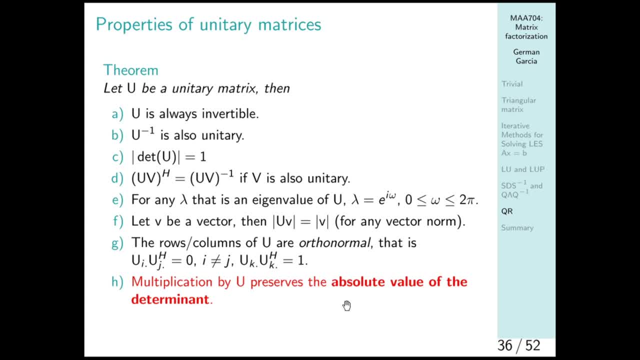 and the same with the rows. And this is one of the most important ones. Multiplication by U preserves the absolute value of the determinant. We know that the determinant is preserved by products. I mean the determinant of the product is the product of the determinant. 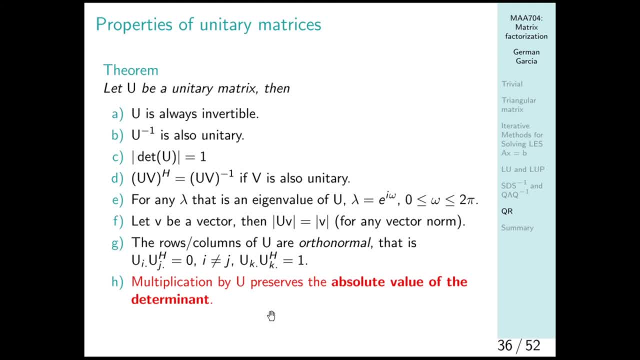 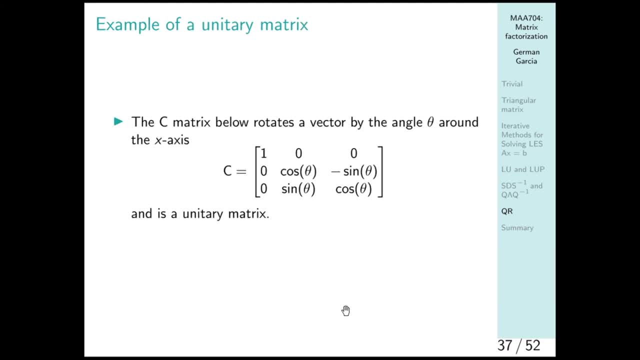 In this case the absolute value of the determinant is one, but this means that the absolute value of the determinant of any matrix times a unitary matrix is kept is preserved. Example of unitary matrix: Rotation of angle theta over the x-axis. 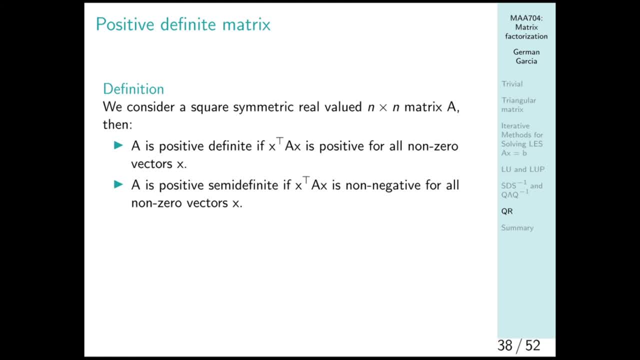 Now consider a square symmetrical real-value square matrix. And okay, do I have a definition for no, All right, So a is positive definite if vector transpose times matrix. times vector is positive for all non-zero vectors and is positive semi-definite if vector transpose times a times x is non-negative. 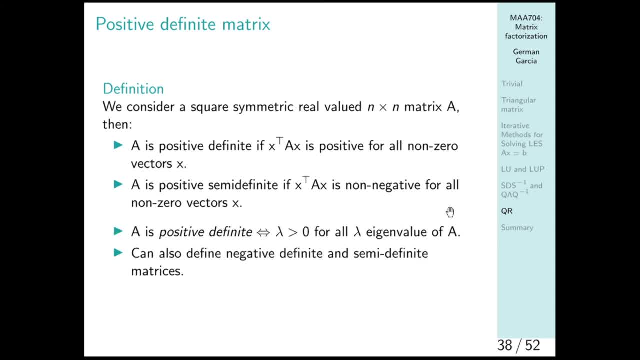 for all non-zero vectors, In this case in the same following. following that logic, this actually implies that a is positive definite, if only if all all their eigenvalues are positive, which contribute to this effect. We can use the same way. 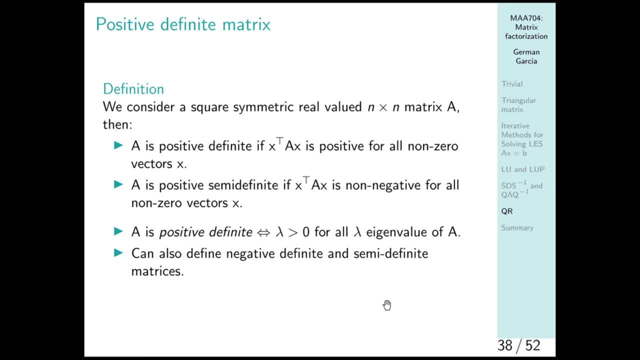 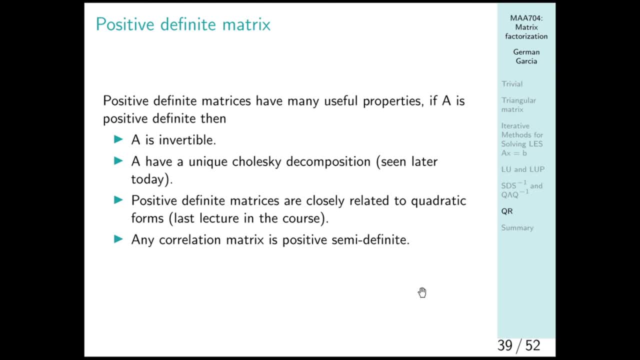 the same thing to to define negative definite and negative semi-definite matrices, and this is going to be an important concept. Now, important properties of positive definite matrices: They are invertible, They have a unique Cholesky decomposition, They are very 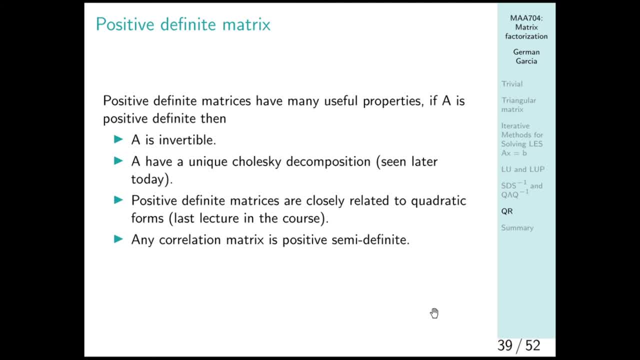 very closely related to certain applications named as quadratic forms that you will see in the last lecture or maybe in the in the last two ones. And lastly, every correlation matrix is positive semi-definite. This is extremely important, especially in statistics. 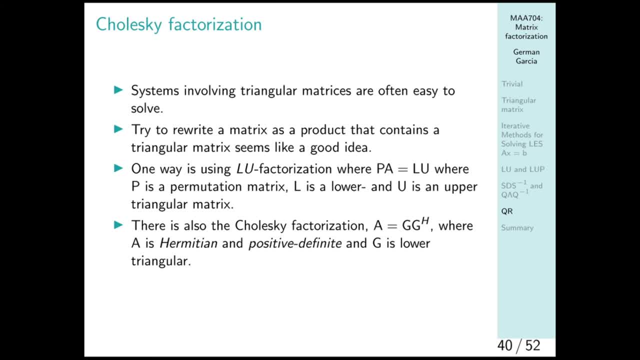 Now, what is Cholesky factorization Systems involving triangular matrices? you know that we are. we can solve them with ease. So dividing the matrix into the product of two triangular matrix is kind of an intuitive way. But we have also the Cholesky factorization. 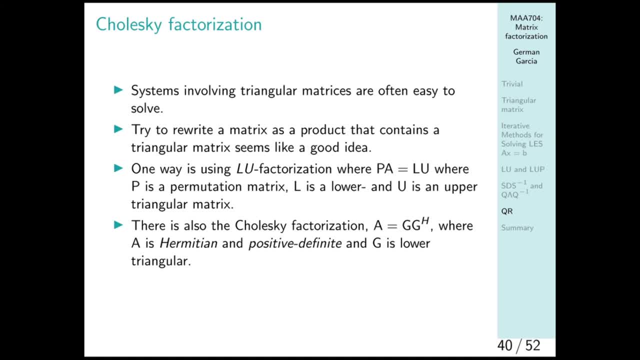 We look for a Hermitian matrix such that A can be expressed as the matrix times its conjugate transpose. The thing here is that we require A to be both Hermitian and positive definite, And in this case G for even more advantage. 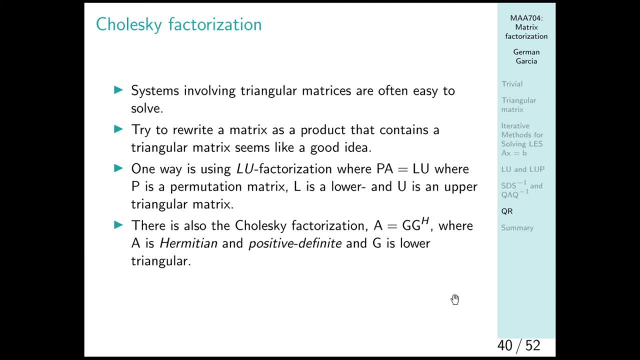 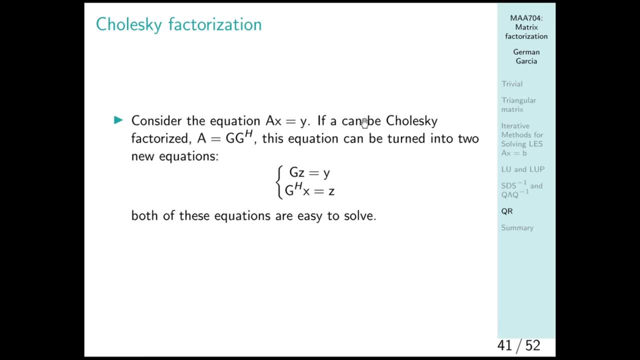 is lower triangular, which makes this upper triangular. So consider the equation AX equals Y. If A admits a Cholesky factorization, A equals G times G Hermitian. this equation can be turned into these new equations which we have already discussed before. 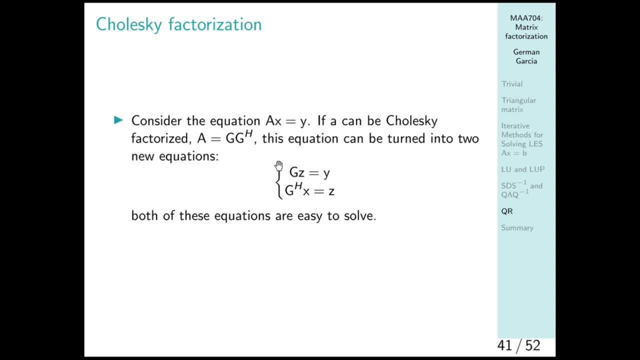 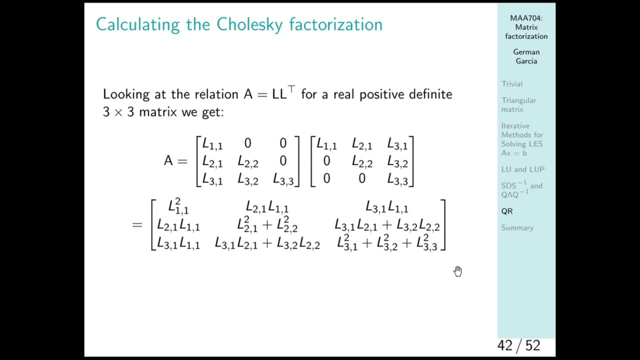 We first solve GZ equals Y and get the value of this vector Z, and then we can substitute here and solve this triangular system. that is extremely easy. For example, if we want to create this, assume that we have that we have real. 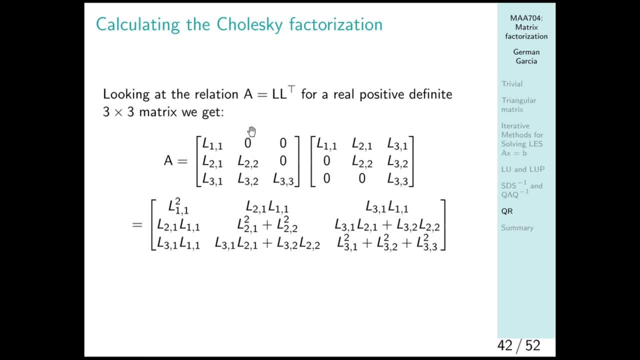 we have real values here, all these elements are real and we're going to see what happens if we brute force our way into that. So we assume that this matrix has to be the product of a lower triangular times its transpose, and what we have is: 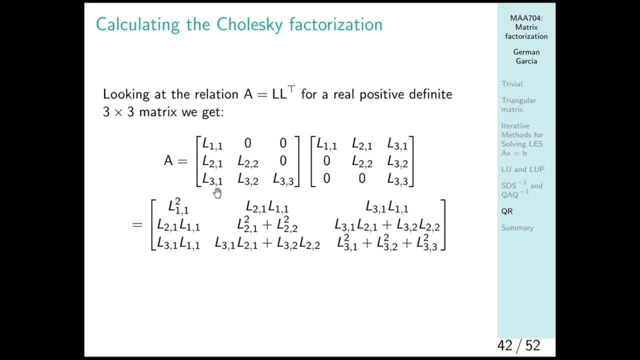 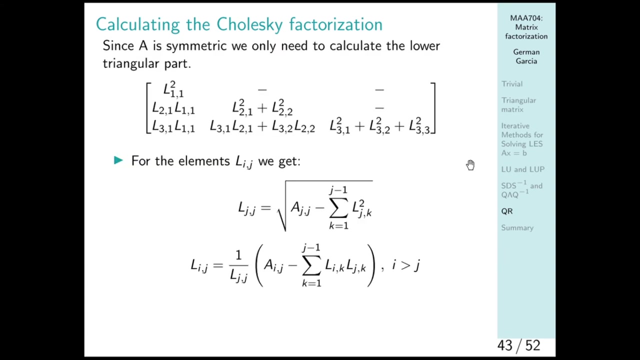 it has to follow this, this form which, once you look at it, this is positive, this is positive, this is positive and, of course, it's symmetric. So this is really convenient And the good thing and the reason why this is so convenient. 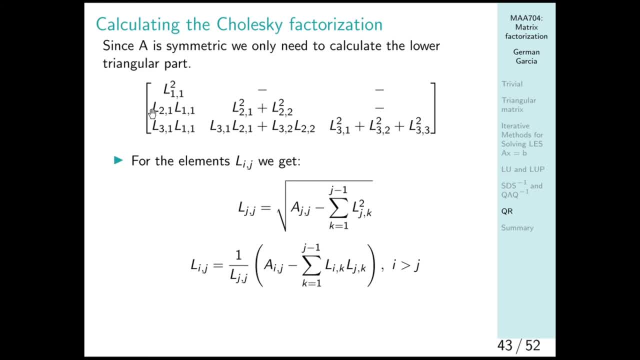 is that we only have to calculate the lower triangular part And see what are the values. So for the elements here we have this. we just try and substitute them into matrix A and we have this, this big monster here, and this. 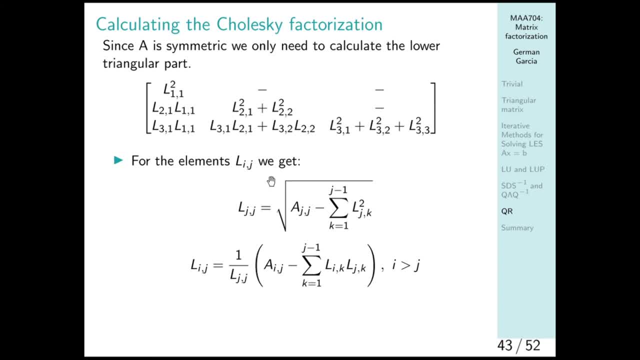 and this little monster here. This is for the diagonal elements and this is for the non-diagonal elements. The trick here is that you might think, hey, but this involves elements we don't know. No, it doesn't. If you want to calculate L11,. 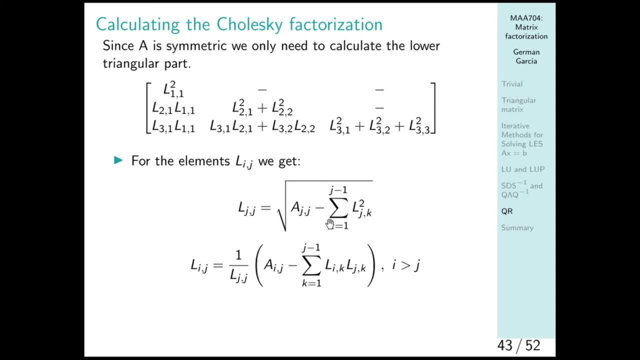 for instance, this is A11 times the sum from k, equal one to zero. so minus nothing, And so we already have this. this L11 will be equal to A11, the square, and when we square it here, we get A11.. 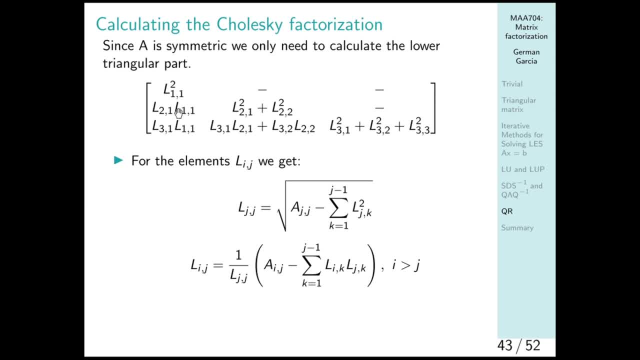 And what we are doing is go one step down and one step to the right, Then one step down, two steps to the right. So we use the elements that we already know to build the new ones Here. L21 involves L11,. 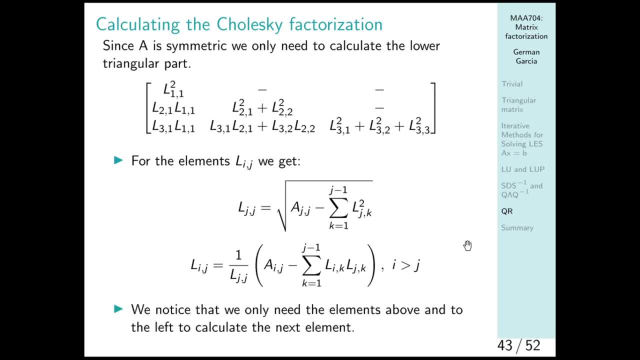 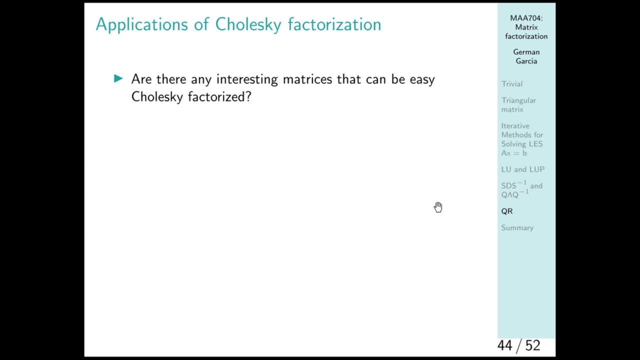 and so on and so forth. So this is the important part of the process. This looks a bit more hefty, but once you get into it it's really intuitive. But now the two questions: Are there any interesting matrices that can be Cholesky factorized with ease? 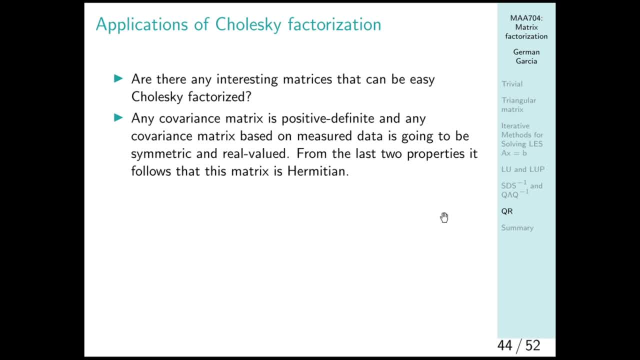 Well, for instance, any covariance matrix is positive definite, And any covariance matrix based on measured data is both symmetric and real-valued, So it really has everything we need. The matrix is Hermitian and so we can use it. We can use Cholesky factorization on it. 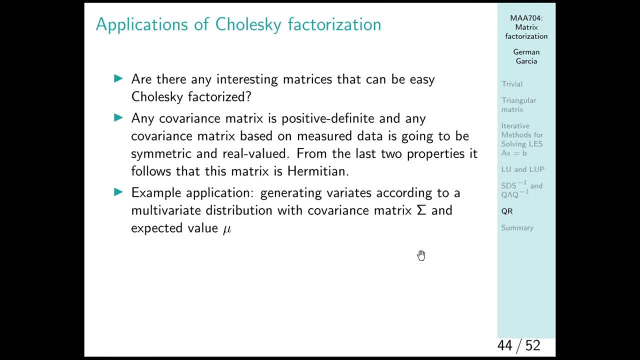 For example, if we try to generate variates according to a multivariate distribution with certain covariance, matrix, sigma and this expected value, we use the Cholesky factorization and our variate is actually the mean plus our Cholesky matrix transpose times the vector of a standard normal variate. 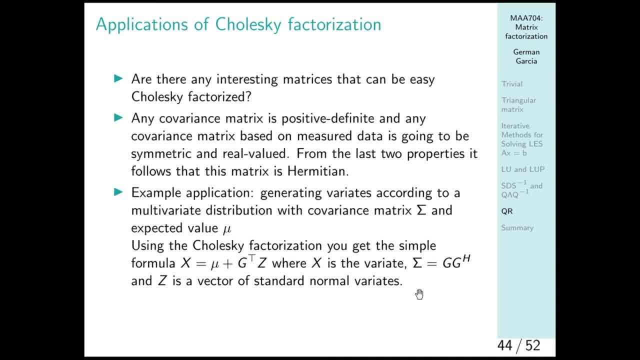 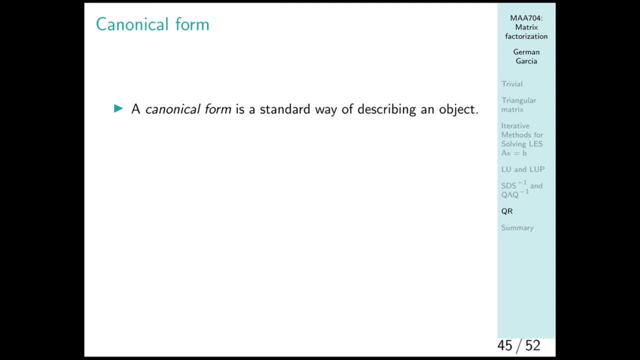 This is huge. This is actually huge. Now I've talked about Jordan canonical form and other canonical forms. What's a canonical form? A canonical form is a standard way of describing an object- anything really. There are several kinds of canonical forms. 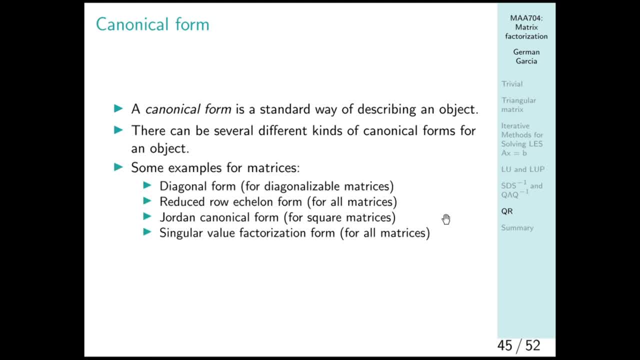 They're usually called normal forms as well. It depends, But generally diagonalized whole matrices. the canonical form is called diagonal form And all matrices can be reduced into reduced row echelon form. I almost don't say it. We have Jordan canonical form. 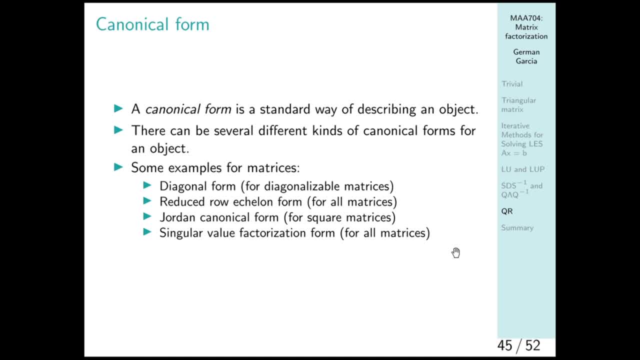 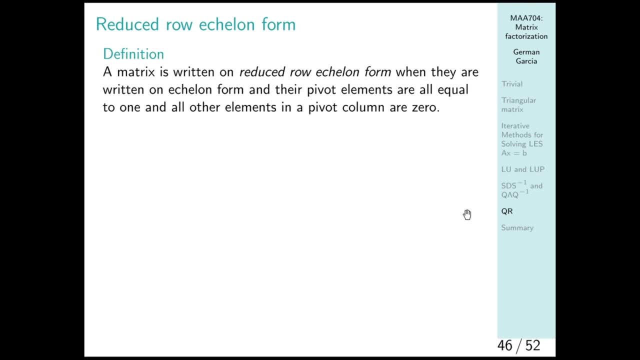 and for a different factorization that we will now see. we have singular vari factorization form. Now, what is reduced row echelon? We say a matrix is written around reduced row echelon form when they are written on echelon form and their pivot elements are equal to one. 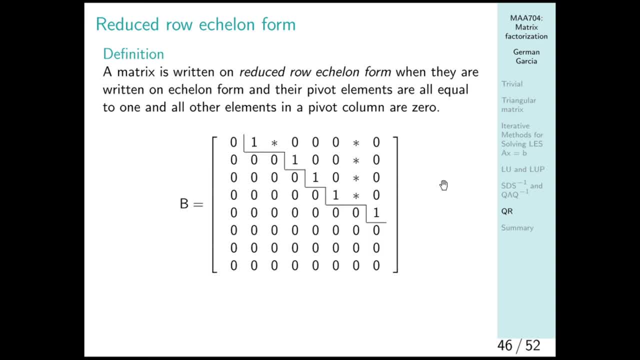 and all the other elements in the same column are zero. Namely, this is reduced row echelon form. Every matrix admits this, And well, this is it. All matrices are similar to some reduced row echelon matrix, If you want to see it in this way. 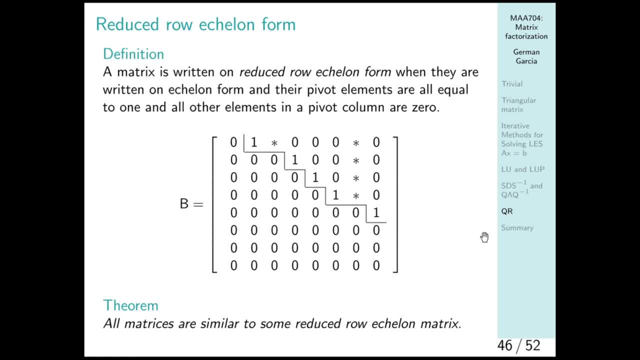 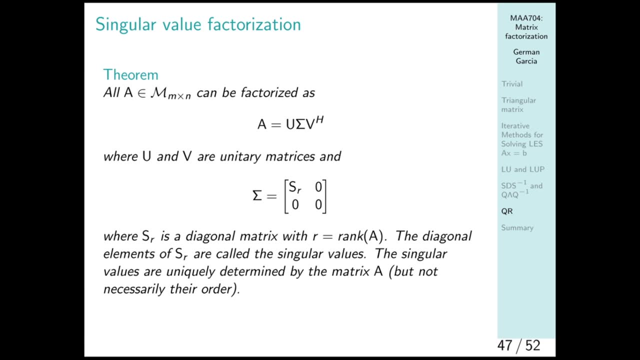 the identity matrix is in reduced row echelon form, So any diagonalized whole matrix that you could think of is actually similar to that. Now, regarding singular value factorization, every matrix can be factorized as a matrix that is part diagonal and part zeros. 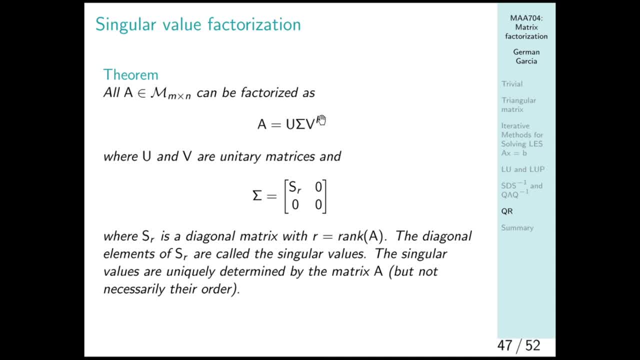 times a unitary matrix, times the conjugate transpose of another unitary matrix, Here R is. this matrix is as big as the rank of A. The diagonal elements here are called singular values and this is what is called singular value decomposition. These are uniquely determined. 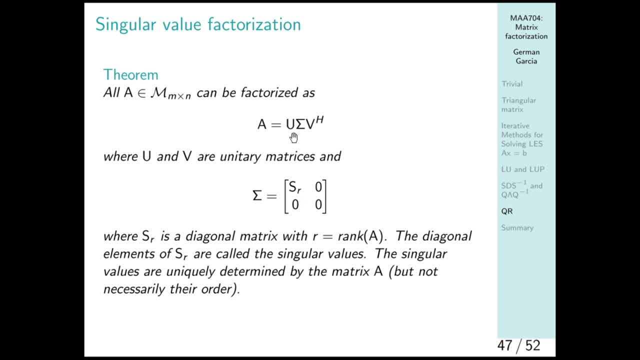 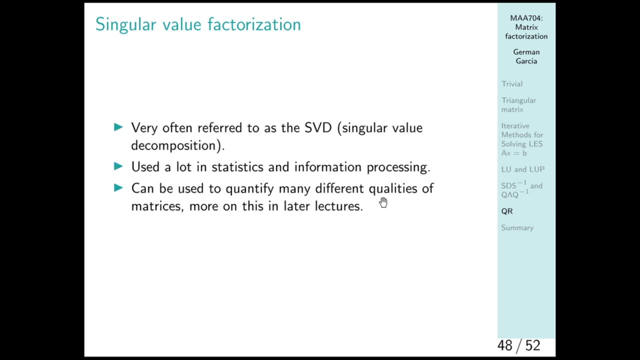 but the order doesn't have to. In certain permutations on U and V, sorry permutations on A- if you permit U and V, you have problems. you can change the order of the values here. This is also called singular value decomposition. 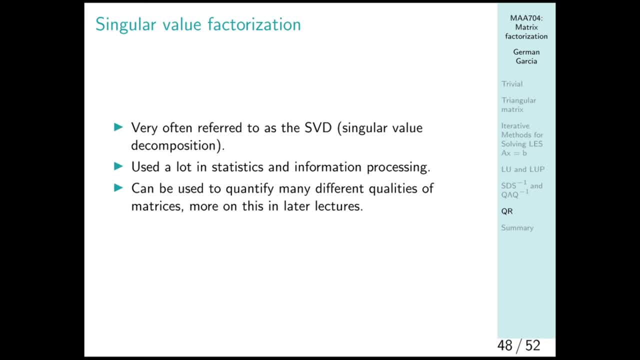 as we will see all the time. It's very common in statistics because it's pretty easy and it gives a lot of precision actually And it can be used to quantify many different qualities of matrices, as we will see. I mean, you will never get tired of SVD. 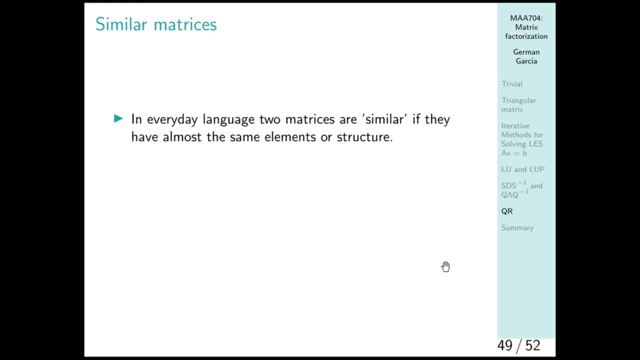 Now we've talked about singular matrices, similar matrices. sorry, Two matrices are similar if they are roughly the same or they represent the same reality from a different perspective, kind of. You can see it in this way: namely, two matrices are similar. 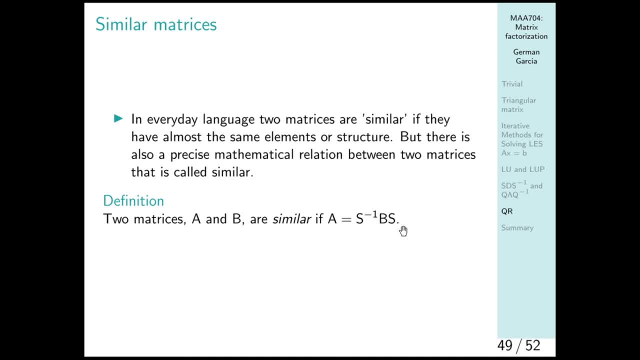 if there is a change of basis that turns one into the other. For those of you who have a strong backtrack in your algebra, S minus one times V times S, this is a change of basis where we will swap the vectors of our elements and look to the matrices. 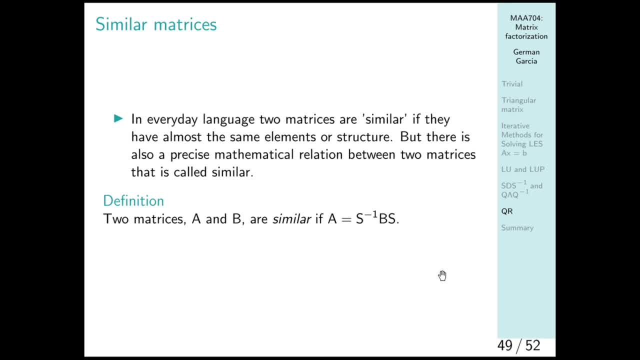 from a different way. The most common use of this is diagonalization, as we have seen, but it can be used to see whether or not two matrices are similar. Of course, the change of basis thing only works for square matrices. Please don't try weird things at home. 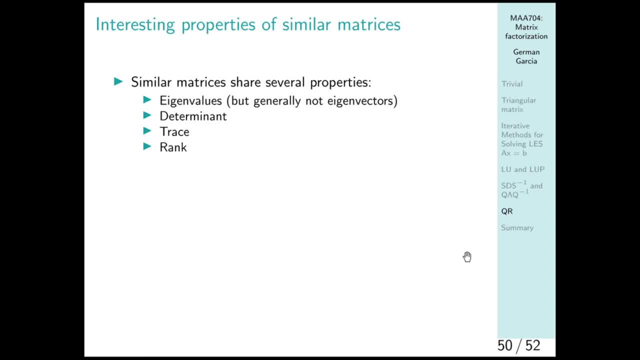 So similar matrices have several common properties, namely eigenvalues, although not eigenvectors. They have the same determinant, they have the same trace, they have the same column, rank or row, rank or rank, And three examples we have seen are diagonalizable matrices. 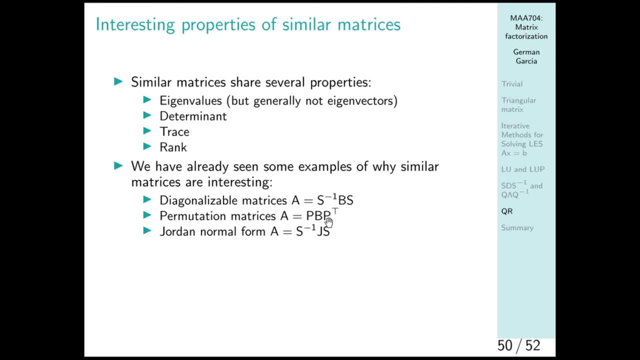 permutation matrices. you may be wondering, but the transpose of a permutation matrix is not its own inverse. It is its own inverse. I encourage you to try and prove it. We have Jordan Normal Form. Any Jordan matrix is, of course, similar to the matrix it is Jordan Normal Form of. 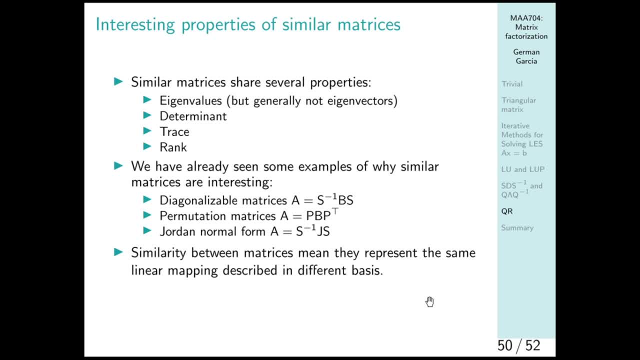 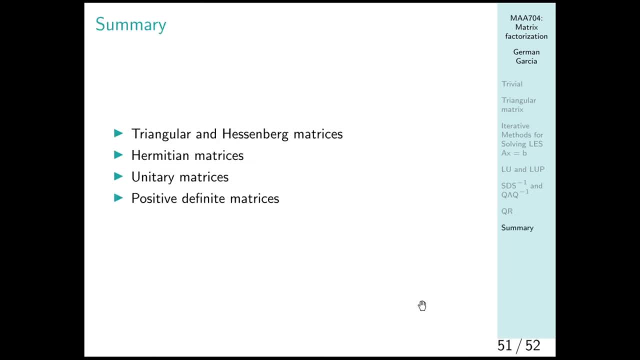 And so yeah, basically similar matrices represent the same linear map roughly. So what have we seen today In a few words? we've talked about triangular matrices, Heisenberg matrices, we have talked about its importance, hermetary matrices.